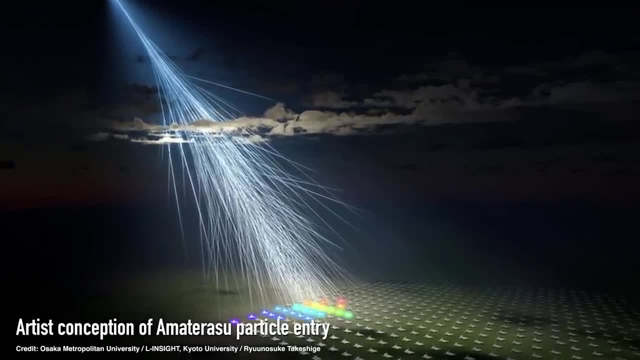 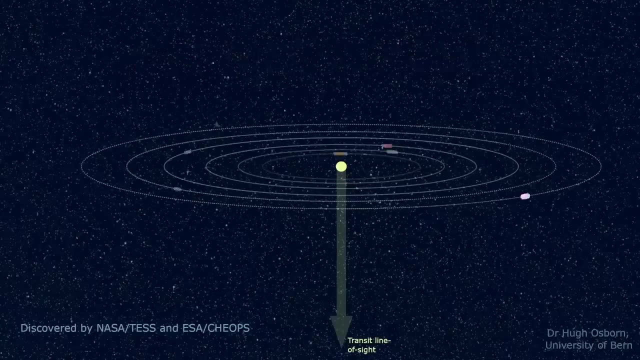 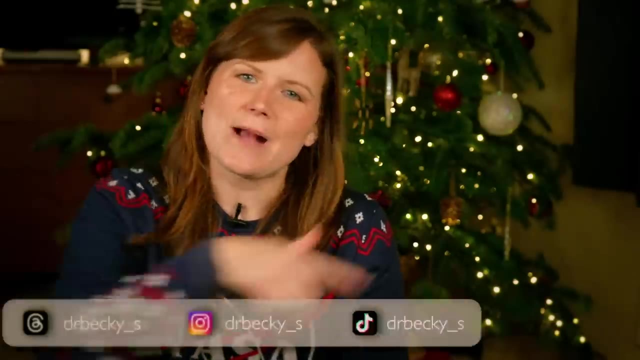 few weeks. In this episode we're chatting about one of the highest energy cosmic rays ever detected, plus the discovery of a six planet system which are all in perfect resonance with each other, and we're chatting about where all the exomoons are, and much more. There's chapter markers down. 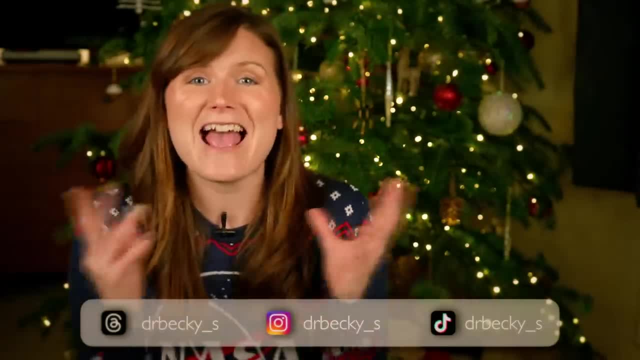 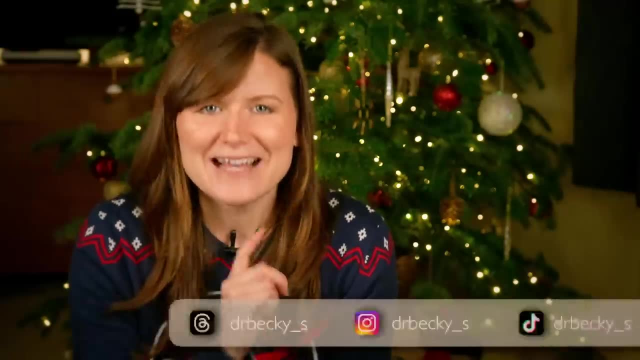 here if you want to skip ahead to any of those specific news stories, plus any scientific research papers I mentioned are all going to be linked in the video description down below, free to read. So, without any further ado, let's kick things off and start by looking up. 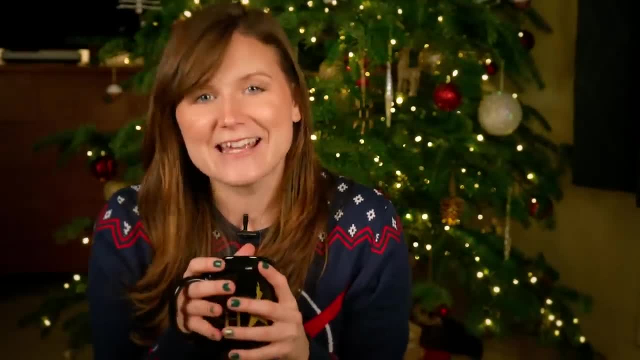 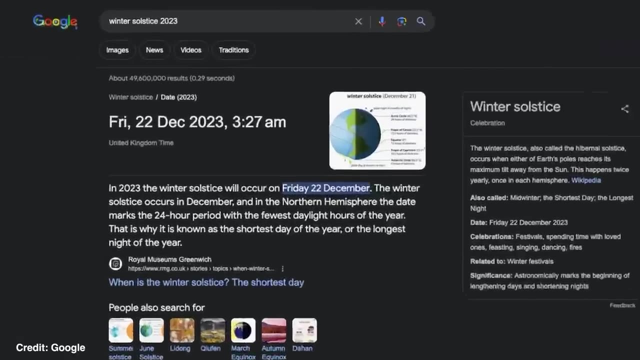 We have officially reached the longest night of the year here in the northern hemisphere with the winter solstice, which this year occurred in the northern hemisphere. It occurs at 3 am GMT on Friday, the 22nd of December. Now if you're wondering how, like the 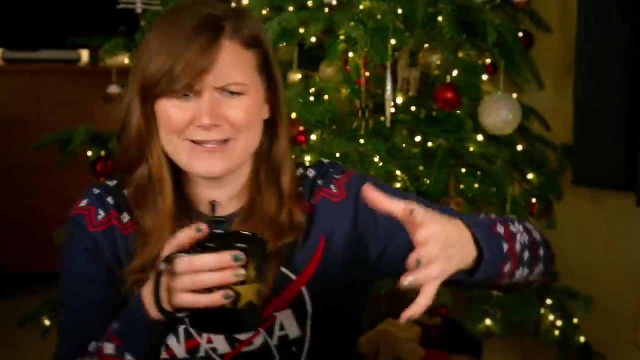 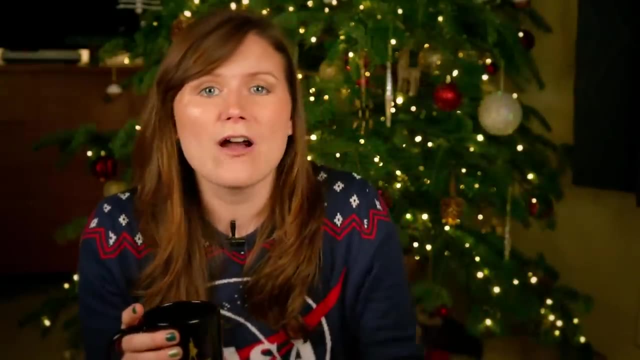 solstice, which the winter solstice is, you know, the shortest day and the longest night- can actually occur at a specific time on that day. it's because the solstice is actually defined by the position of the sun in relation to the background stars. You can think of it kind of like longitude, but 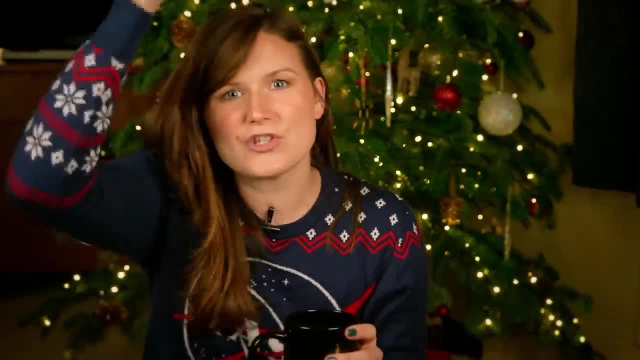 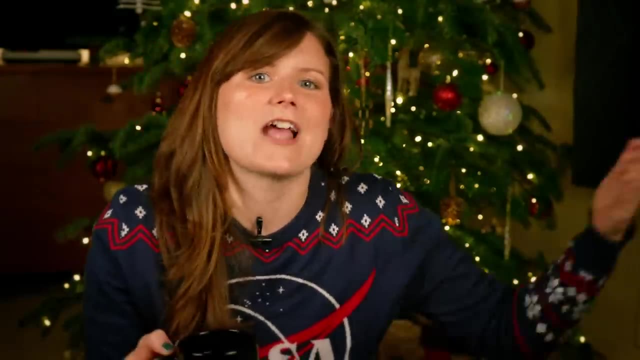 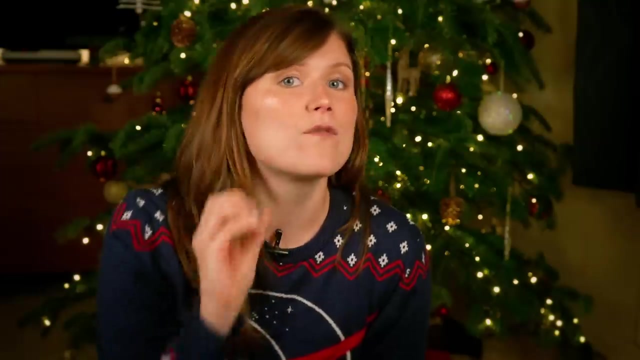 on the sky. so like zero degrees longitude, you know, as GMT runs through London, zero degrees longitude degrees on the sky is where the sun is on the March equinox, when you've got equal day and equal night, and the winter solstice is when the sun is 270 degrees around. from that position, What it 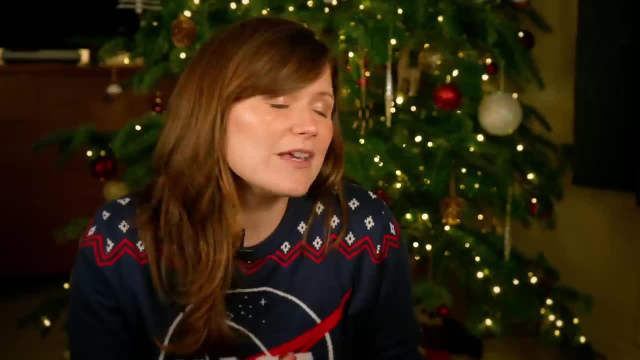 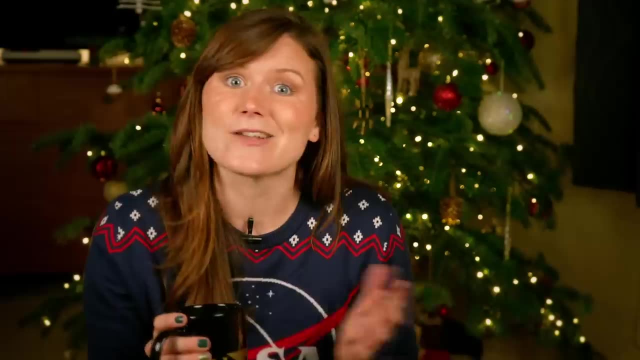 essentially means for those of us up in the northern hemisphere anyway, is that we have got incredibly long nights that we should take advantage of to stargaze while we can, because the nights are only going to get shorter from here on out. So, on the nights of the 21st and 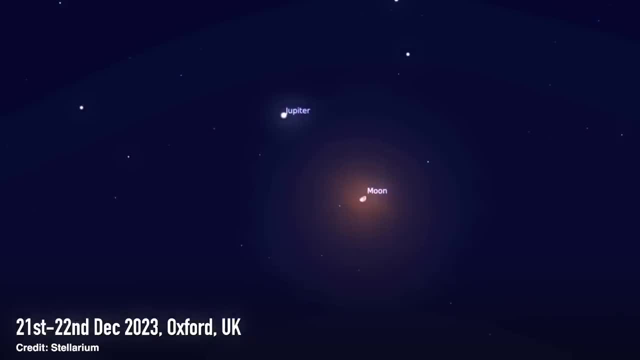 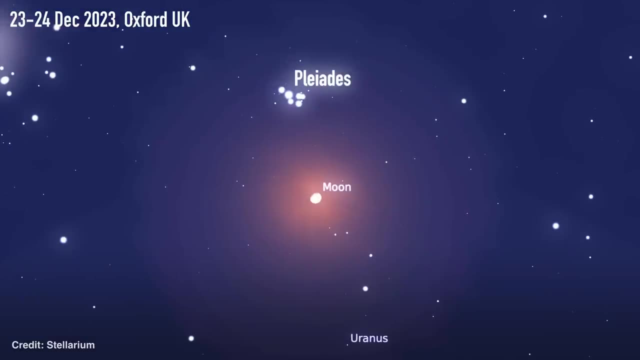 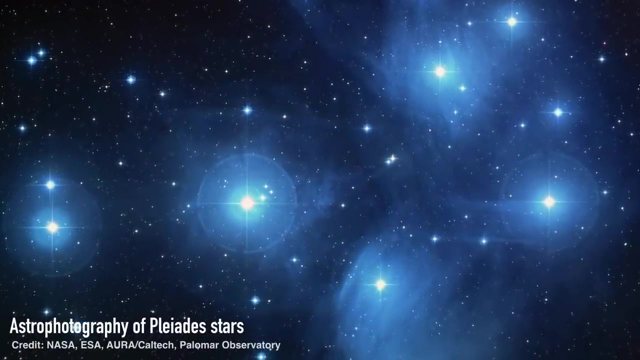 22nd of December, the just past half moon will be close to the planet Jupiter on the sky, before then moving closer to the Pleiades star cluster on the 23rd and 24th as the moon gets closer to becoming a full moon. Pleiades is the one that looks like a little mini, big dipper or plow. 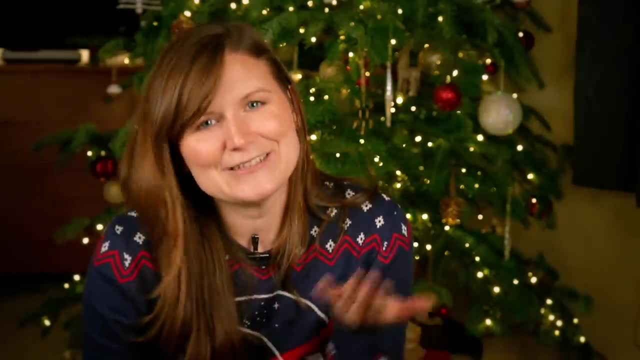 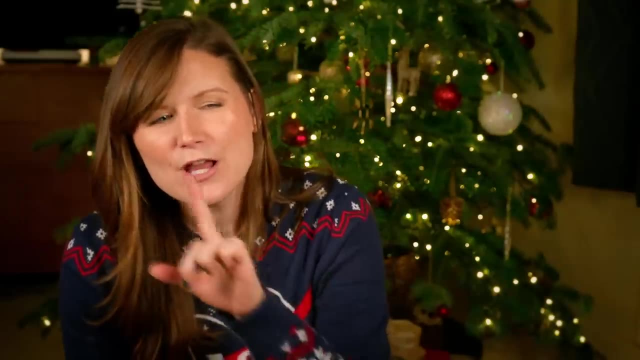 constellation, and it is one of my favorite things to look at in the winter sky. Once you've spotted it, your eyes will always find it again. it's just beautiful. Now the moon will be in the very bright because it's getting close to full, so it will wash out a lot of the stars that you 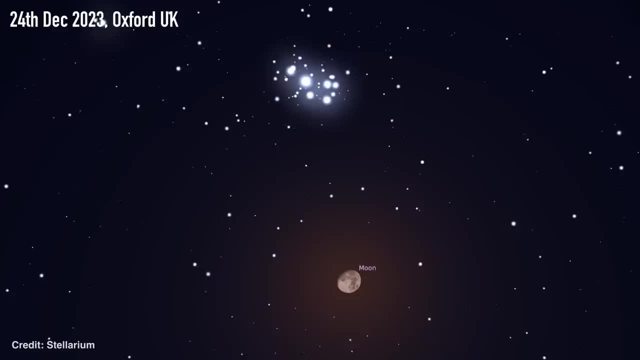 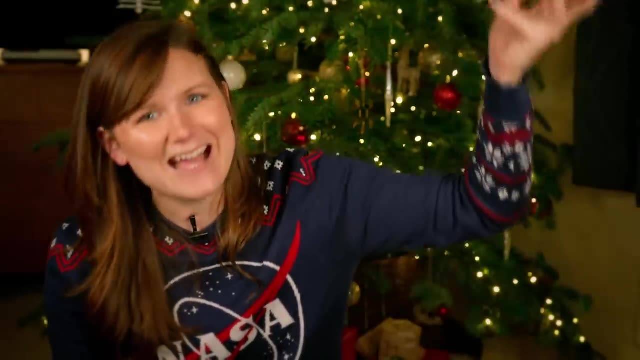 would otherwise see if you look at Pleiades with binoculars or a telescope. But if you're not sure where to look, it is just a good trick to find things like Pleiades and Jupiter on nights, where the moon is there, so that you know where they are in relation to you. know things in your back garden. 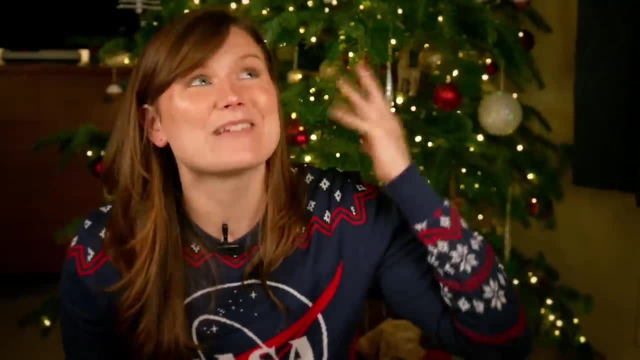 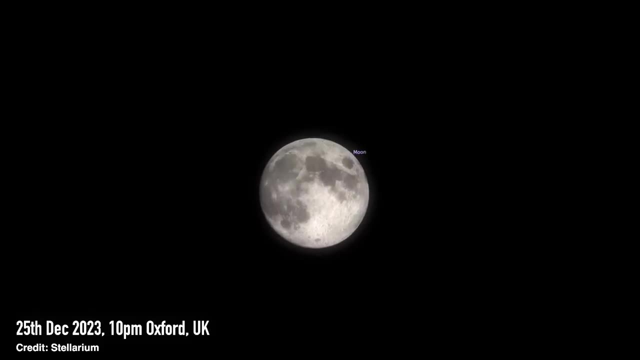 you can come back another night when it's much darker and look again, because this part of the sky is incredible. during the winter. it just feels like there's so much going on. Plus, by the night day, the almost full moon is going to be smack bang in the middle of the winter hexagon that I talked. 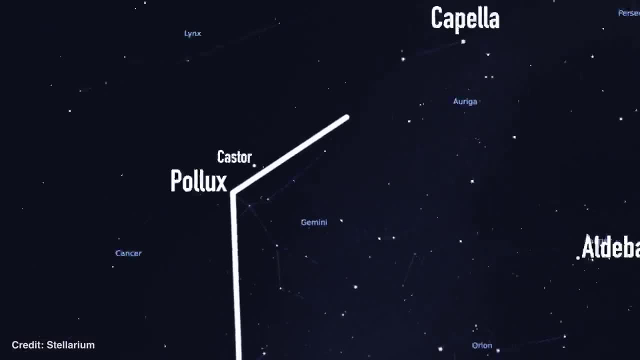 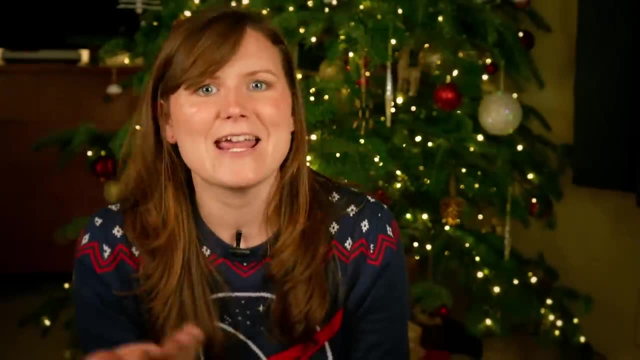 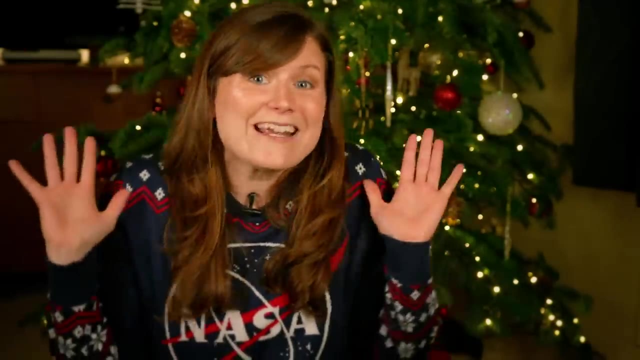 about last month, Six of the brightest stars in the winter sky that are a sight not to be missed. Also, if you have clear skies on either Christmas Eve or Christmas Day morning, look out for the International Space Station passing overhead where you live, because I give this warning every year to 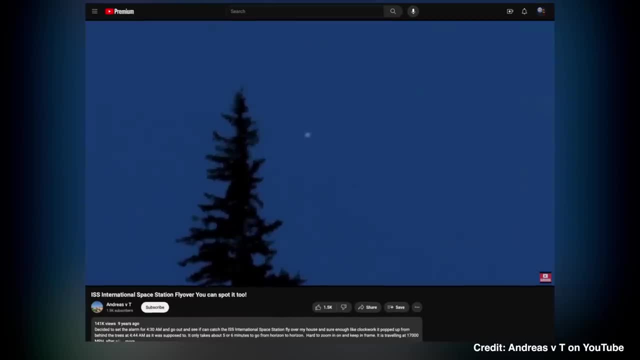 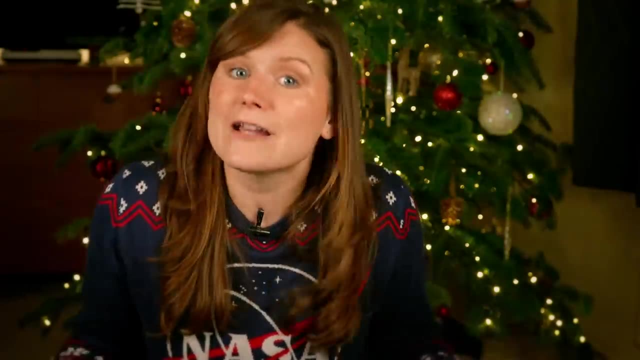 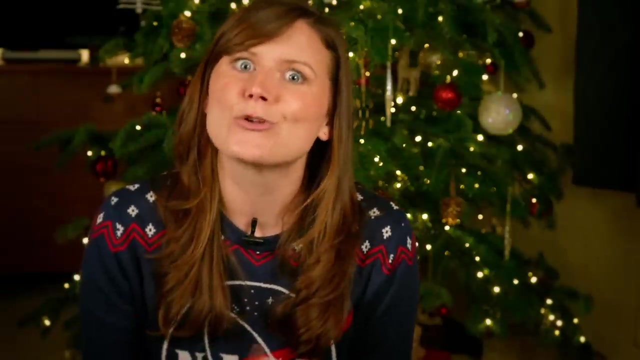 parents of kids out there, because the International Space Station can look very convincingly like its father Christmas's sleigh. you know it moves very fast and it's incredibly bright. so you know, I just I wouldn't want any kids out there to get the two confused. Now, thankfully, 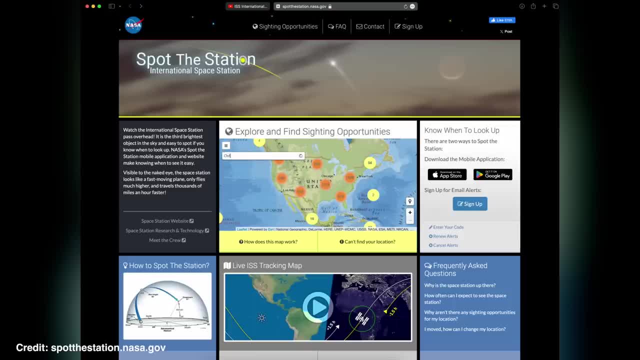 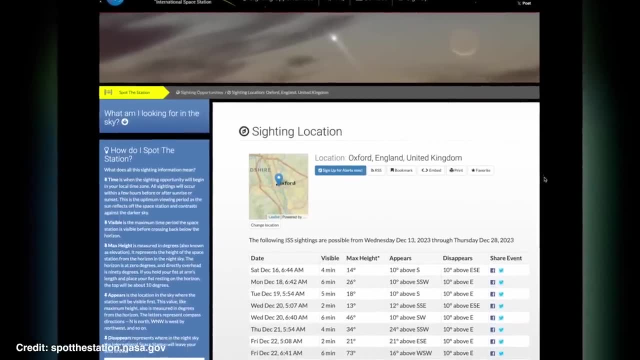 NASA have a helpful website that you can look up when the International Space Station will be passing over where you live and which direction to look in. For example, here in Oxford on Christmas Day morning at 6am, the International Space Station will go directly overhead appearing. 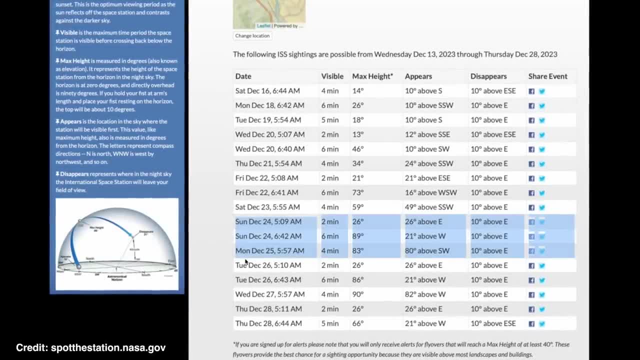 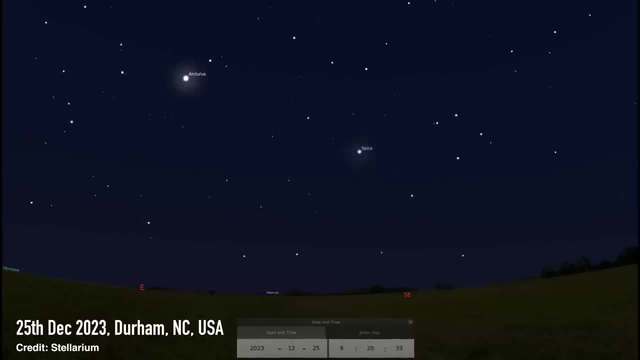 first in the middle of the night, and then in the middle of the night, and then in the middle of the night west, and then setting in the east six minutes later. So if you are up that early anyway, it might be a good thing for the whole family to look out for in the night sky. While you're there, look to. 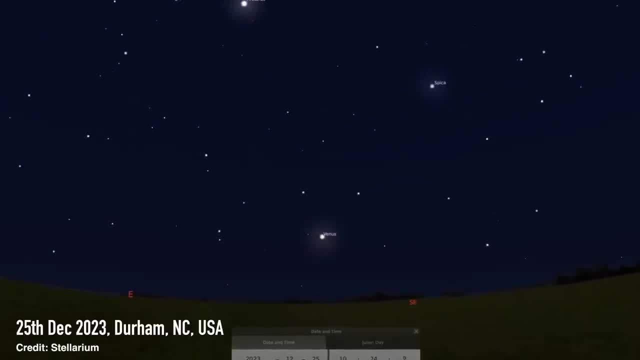 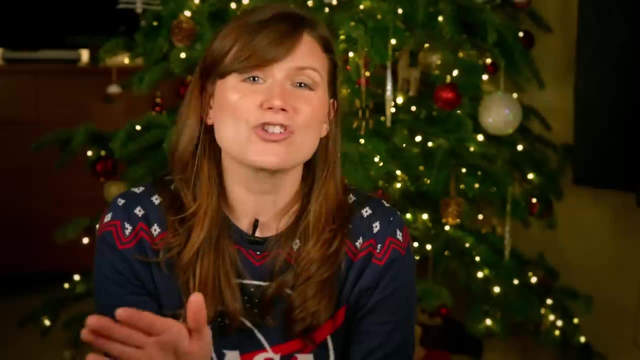 the east for Venus rising in the early morning sky. it's the brightest thing in the sky after the moon, so hopefully you won't be able to miss it as it shines out as a beautiful Christmas morning star. It's not just Christmas morning. you can see Venus, though, like it's visible throughout December, and 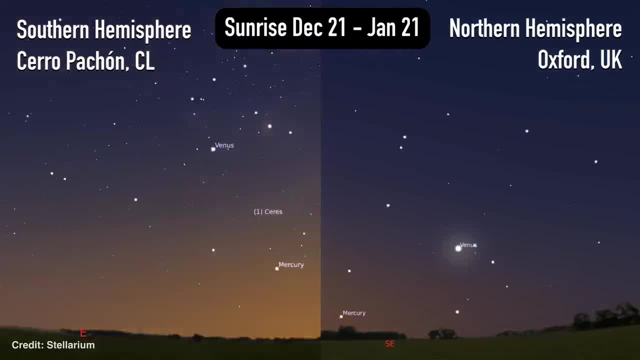 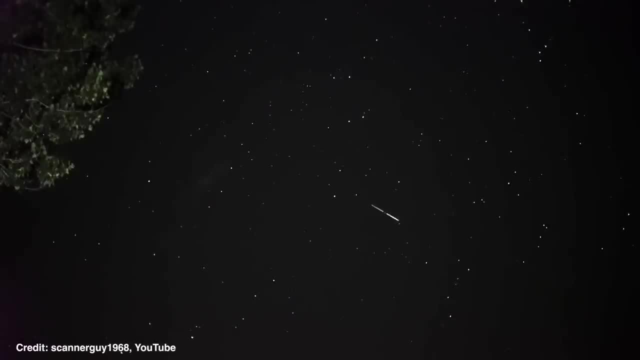 January now. so if you're ever up that early and you've got clear skies, look towards the sunrise in the east and see if you can spot it. Speaking of January, heading into the new year, those of us in the northern hemisphere have got yet another meteor shower to look forward to the Quadrantids meteor shower, which peaks next year. 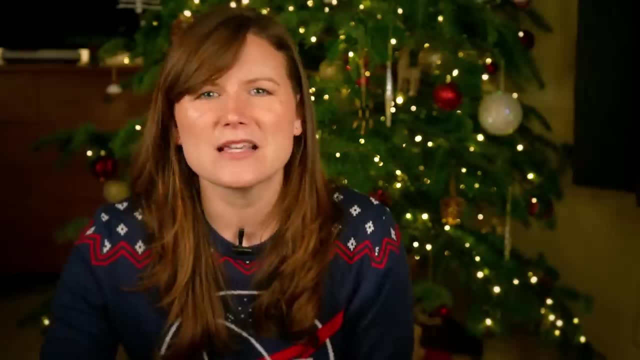 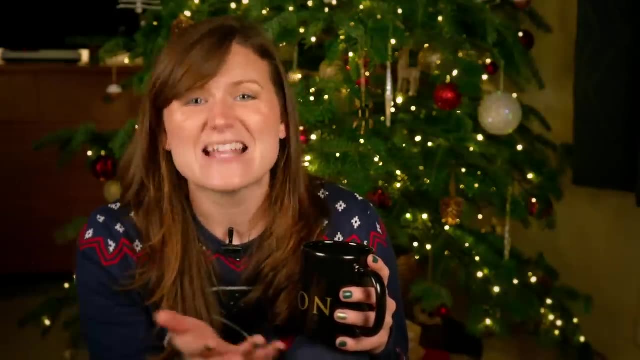 on the 4th of January 2024, but you'll start seeing meteors from like around about like the 28th of December, like right through till the 12th of January. so if you're out stargazing on those nights, just keep an eye out for a few shooting stars. Now, in previous years, on the peak, the Quadrantids has given us about 200 meteors per hour, so they're known to put on a show, but this year best estimates put it around about 100 meteors an hour or so. still a pretty good show, but that's only in the darkest of skies, at the peak at 1am on the morning of the 4th of January. so 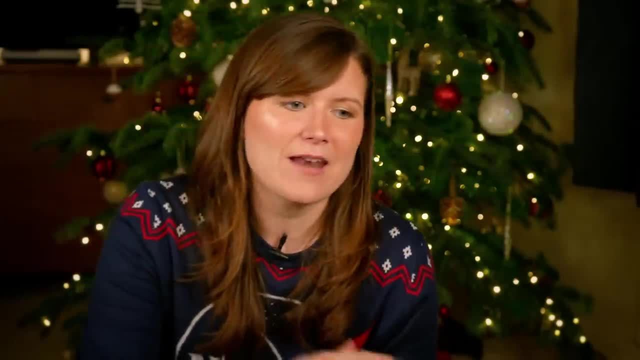 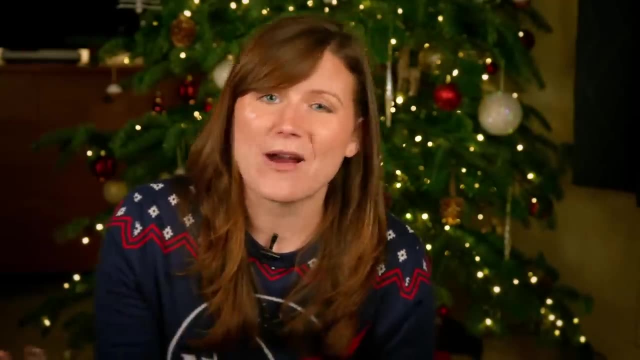 that number of meteors is gonna drop off. you know, depending on a how close to light pollution you are. you know if there's a lot of light pollution, that's going to wash out all but the brightest of meteors, so you will see less of them. and also you know what day you're actually going to see less of. 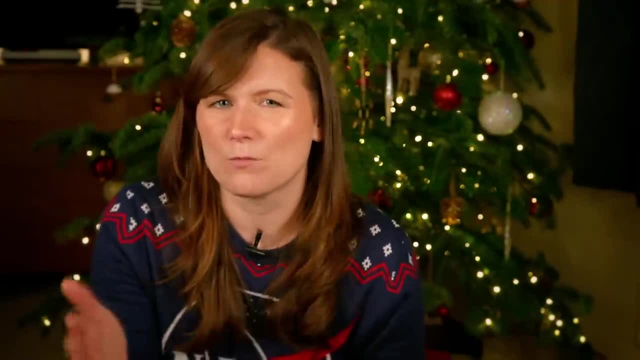 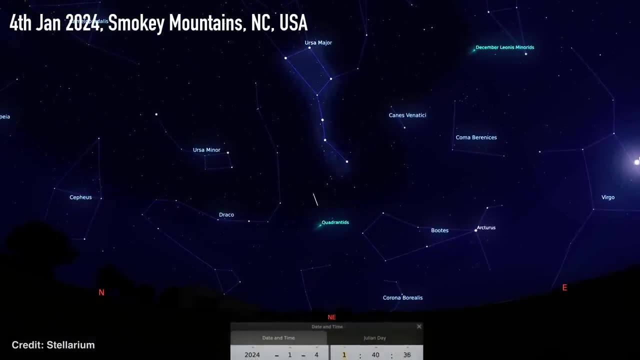 them, and also you know what day you're actually going out to look for the meteors? like, how far either side from the peak are you? The meteors are all going to appear to be coming from near the handle of the plow or big dipper constellation, hence why this isn't one for anyone in the 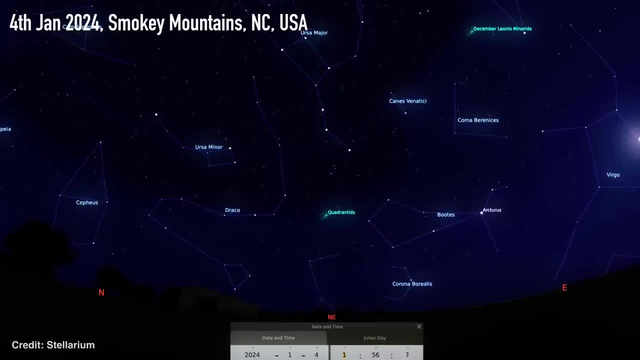 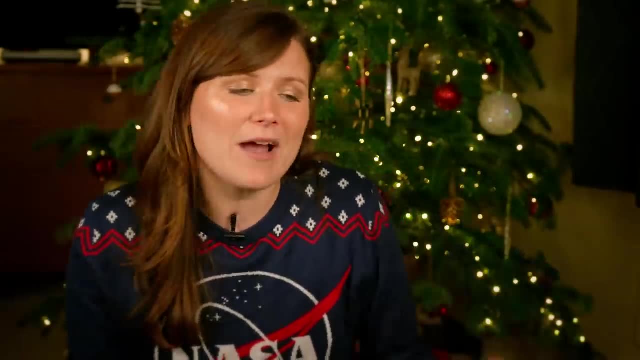 southern hemisphere, sadly, because this is pretty high on the northern sky To spot these. you're essentially going to want to just look anywhere but the plow constellation, because they're going to be streaking away from there. so my advice: just grab a blanket, pop it on the floor, lie down and 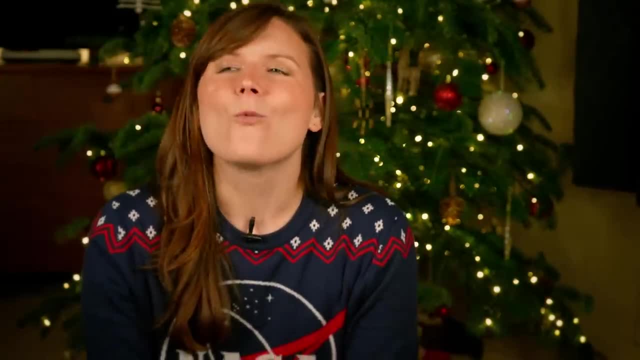 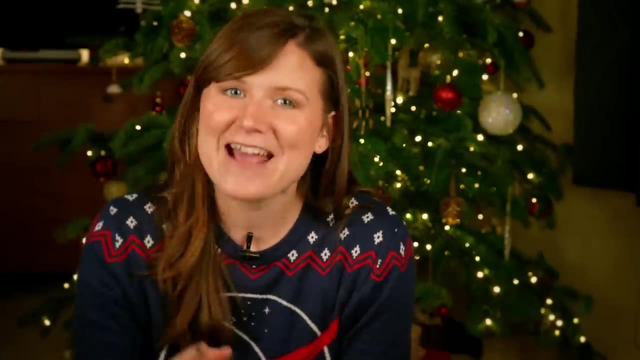 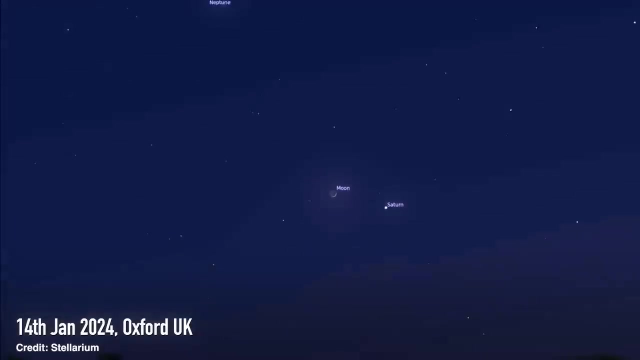 look directly up and enjoy the show. Now one more thing, because I actually don't know if you've seen this, but I absolutely can't resist, because my favorite planet, Saturn, is pairing up with my favorite moon phase, a crescent moon aka the toenail moon, on the 14th of January in the early evening. 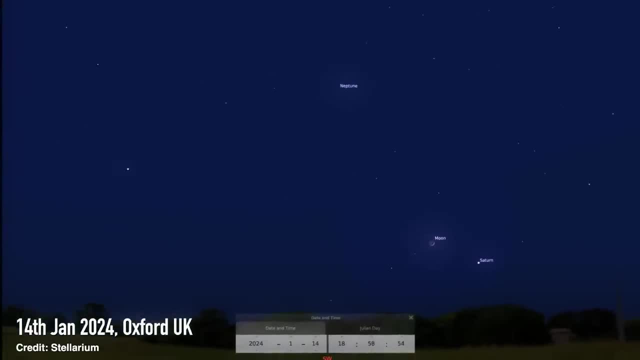 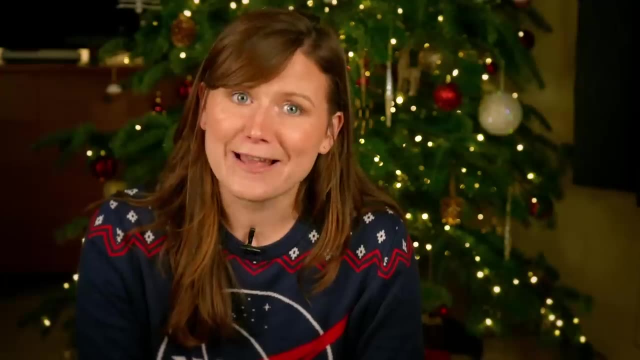 just after sunset, before they set together a few hours later. If it's clear that night, make sure you try and spot this one and also send me a picture on social media if you do, because, let's face it, it's very likely to be cloudy here because Saturn will actually be disappearing from our sky. 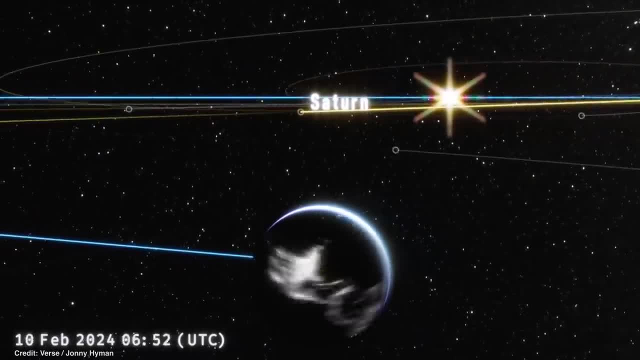 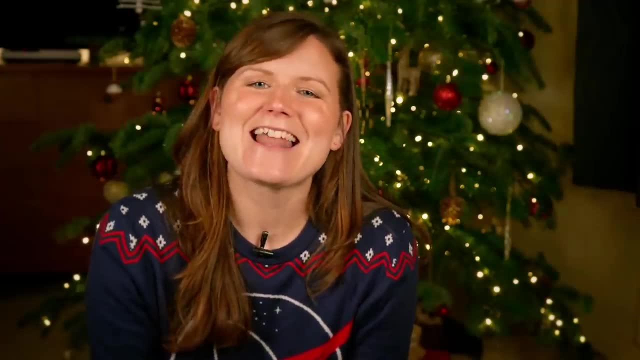 as soon as it gets closer and closer to the sun, From our perspective here on earth, actually swing around behind the sun and eventually reappear in the morning sky in late spring. All right, that's enough of looking up at the night sky. let's come back down to earth now and chat about what's been happening in space news in the 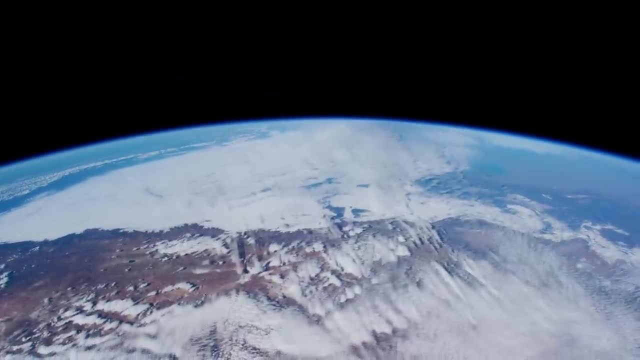 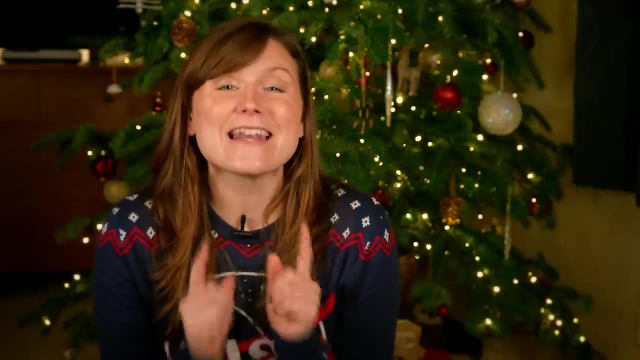 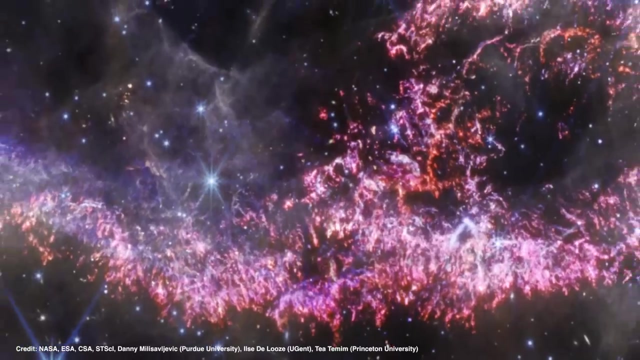 past month. All right, there is a lot to get through this month, but let's start by looking at the latest color image released by NASA from JWST of the supernova remnant Cassiopeia A. This is an image of a star that has run out of fuel and died by going supernova and then throwing off all of its 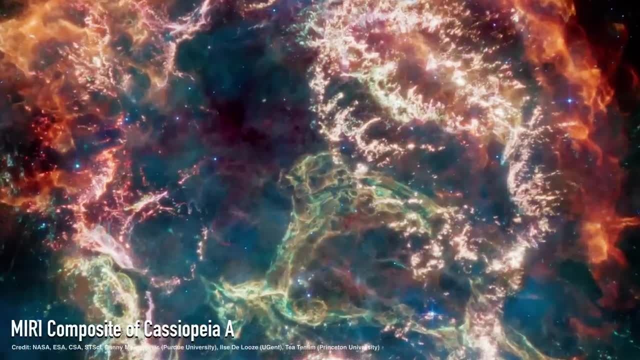 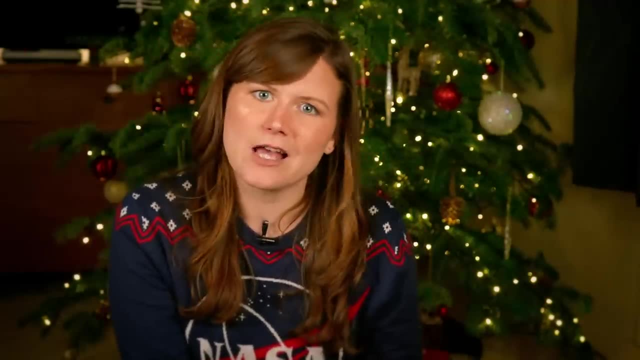 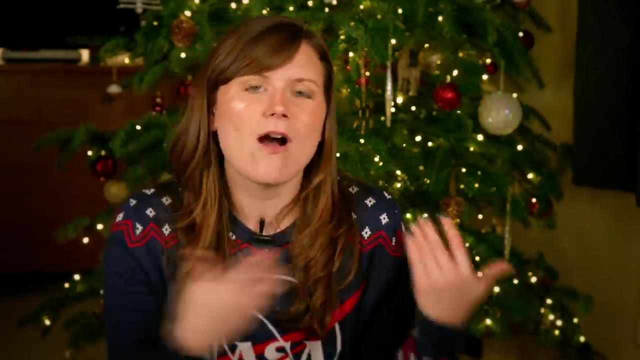 outer layers of gas which are now lit up by the core of the star left behind in the center. Now remember this isn't a real color image because the JWST detects infrared light and not visible light that we actually see in colors. but we do color the images because then your eye can pick up a lot of. 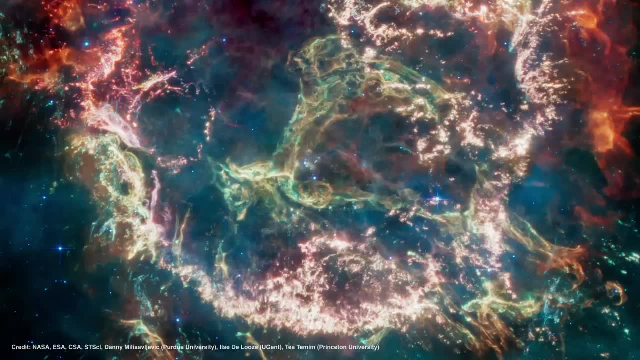 scientific details that it otherwise would miss in black and white. So the telescope takes an image of a star with shorter wavelengths of light given off by hotter regions, and those are colored blue- and then another that only lets through longer wavelengths of light given off by cooler regions. 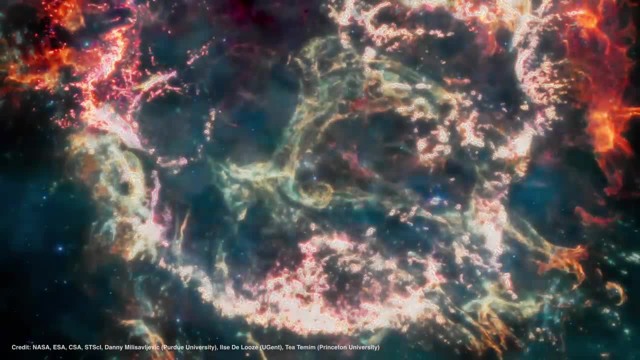 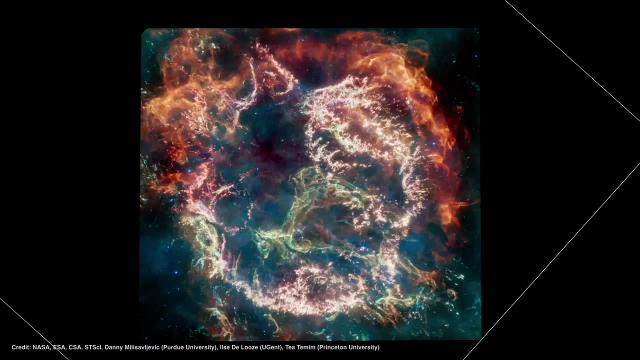 and those colored red, and similarly with middle length wavelengths that are colored green in the middle, and so you can see where gas is hotter and cooler just by looking at this image. I mean, JWST's resolution is incredible right. it can detect these tiny knots of gas here that are made of like sulfur. 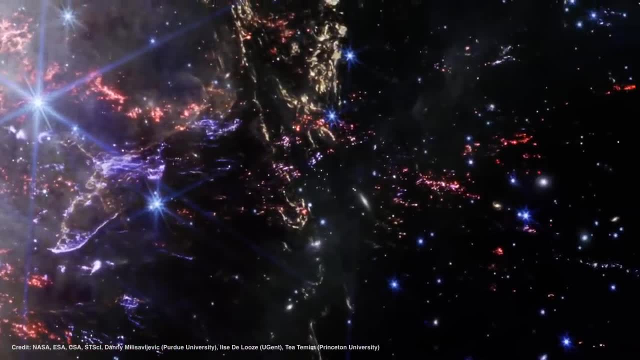 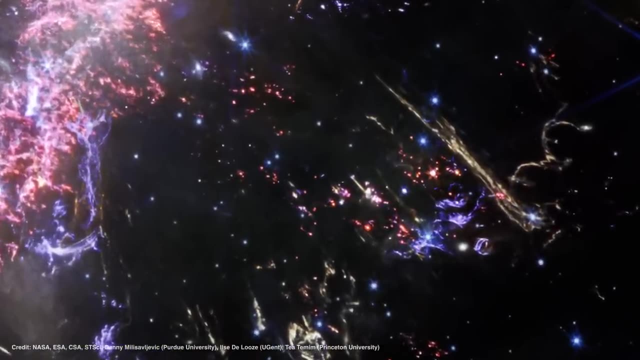 oxygen, argon and neon that have all come from the star itself, and some of these filaments of debris here are two times as big as the star itself. So this is a very interesting image of a star that's tiny even to be resolved by JWST, meaning that they're less than 10 billion miles across just. 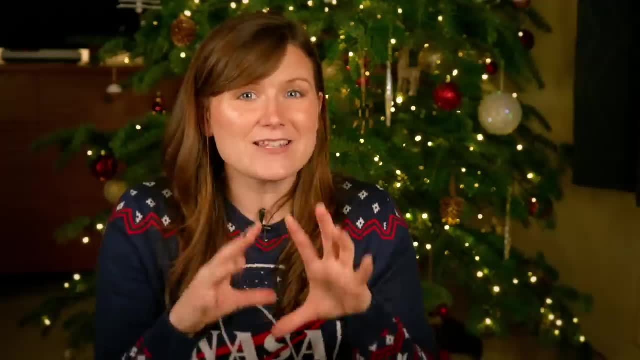 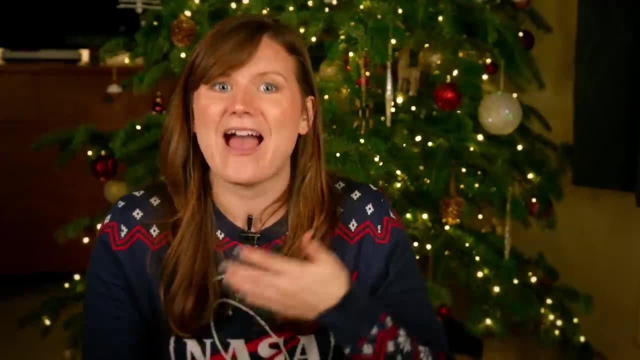 around about a hundred times the distance from earth to the sun. Now that suggests that this star, when it went supernova, essentially shattered like glass. so studying images like this gives us a really good idea of how this process happened, which was the scientific motivation for taking 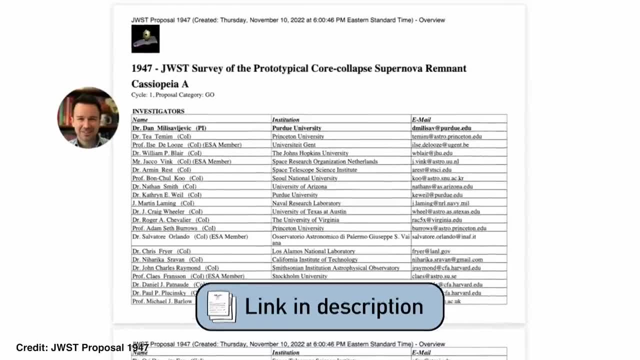 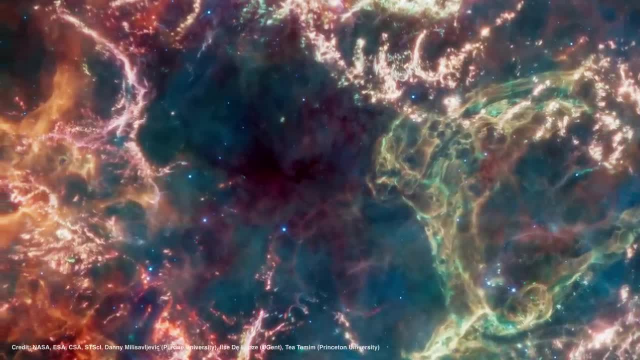 this data in the first place, which was written in this proposal written by Mili Savoljevic and collaborators. So I'm sure we're going to be seeing a paper analyzing this incredible image and all the other data they've collected published very quickly. 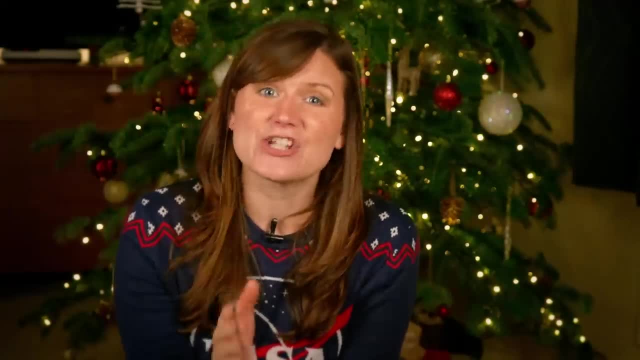 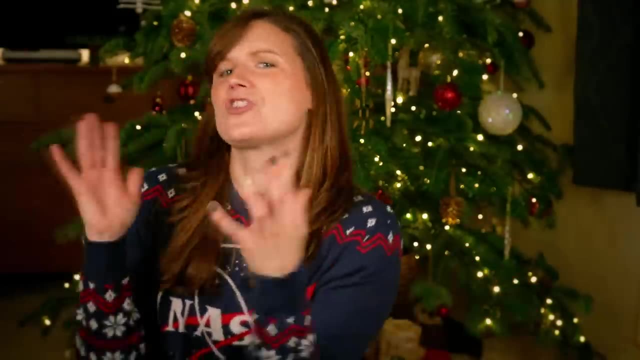 While we're on the topic of space telescopes, Hubble has been having issues with its gyroscopes once again this month. The gyroscopes are part of the system that allows the telescope to know which direction it's pointing in, so they're pretty crucial for the continued operation of the telescope. if you 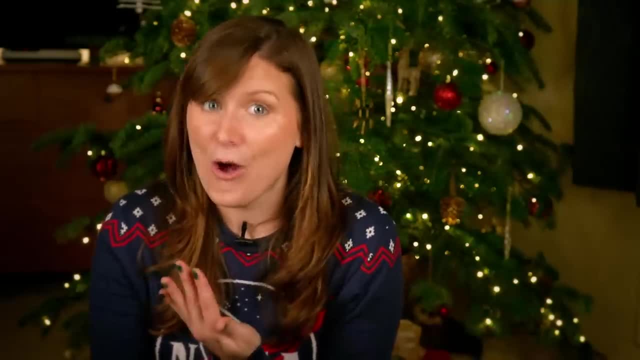 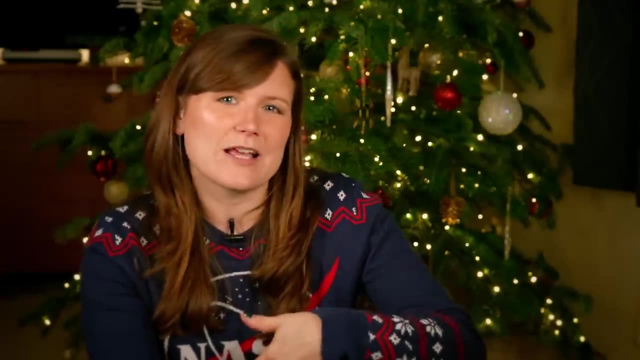 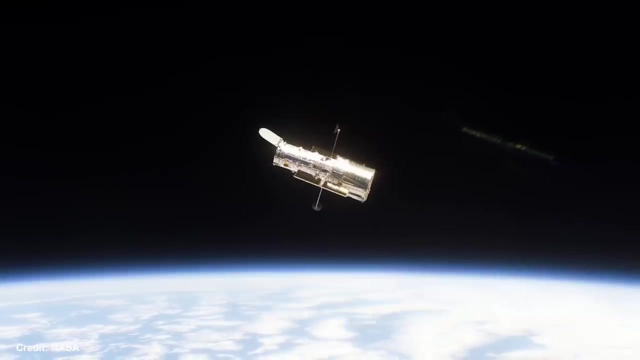 want to look in a specific direction, at a specific object. Now, over the 33 years that Hubble has been operational for the gyroscopes have been replaced a number of times, but you know, the last servicing now for Hubble was over 15 years ago, so we're stuck with the ones that we have now, since there's no. 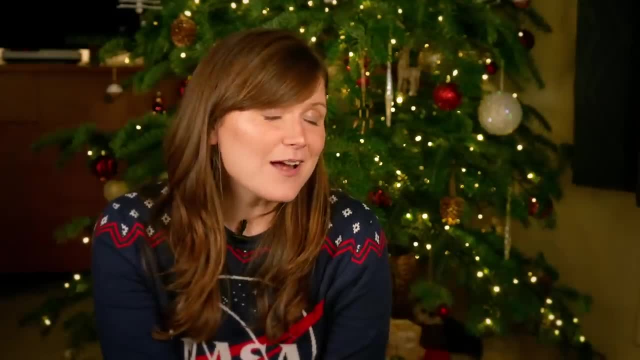 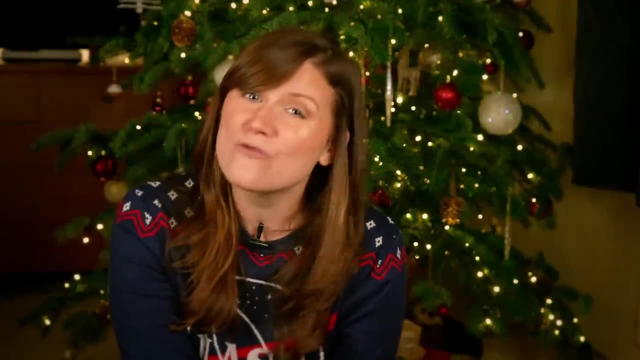 space shuttle that can service it anymore. And now it just seems like every time there's trouble with Hubble it's because of the gyroscopes, you know, which isn't exactly surprising. it's always the moving parts in space that scupper you. So the telescope systems entered what's known as safe. 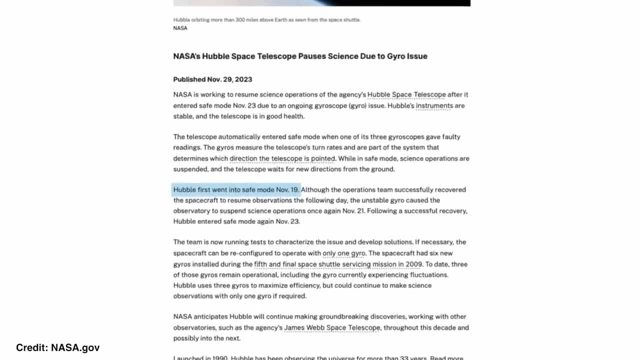 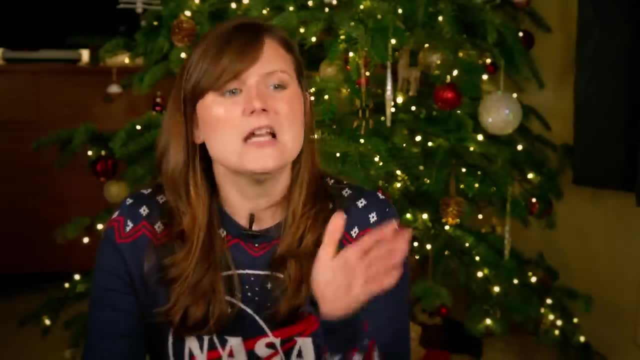 mode on the 19th of November when the problem was first identified, With one of the three gyros on board just giving some strange readings. so you know for safety's sake, or you know if you're going to be able to get the telescope back up and running again on the 21st of November and restarted. 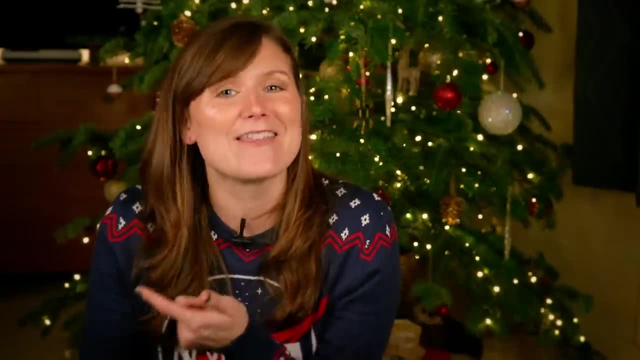 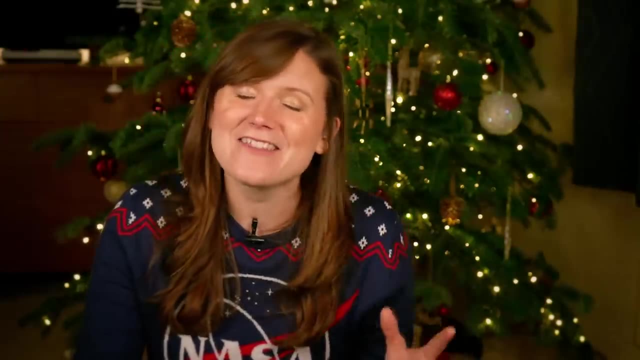 observations, but then the telescope was back in safe mode by the 23rd of November. So the team spent a little bit longer analyzing all of the data from the gyros and have managed to get the telescope back up and running again on the 8th of December and, fingers crossed, everything seems to. 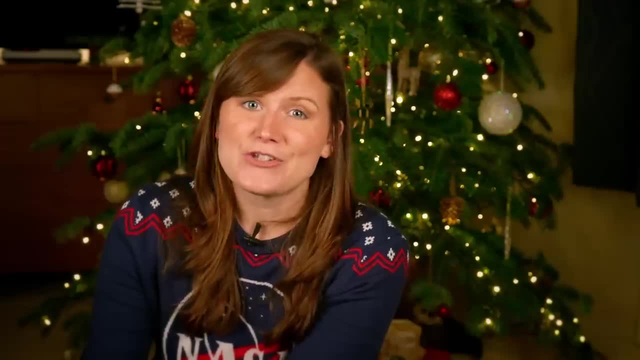 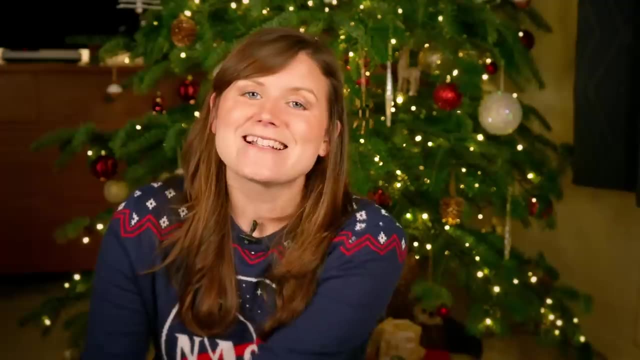 be fine. Fingers crossed, because you know, I'd quite like to put in an application to use Hubble for my next round of proposals that are going to be due in spring that were just announced the other day. But it's likely that as Hubble continues to age, more issues like this are going to crop up. so we're going to have to get used to having some pauses in observations and some people just missing out on the observing time that they were scheduled to have, which is a real shame, But the hope is that Hubble will continue to operate well into the 2030s. 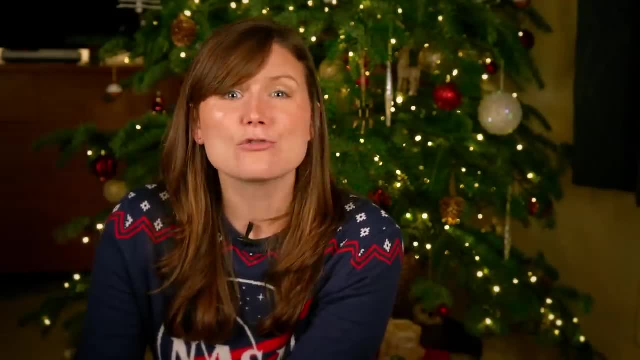 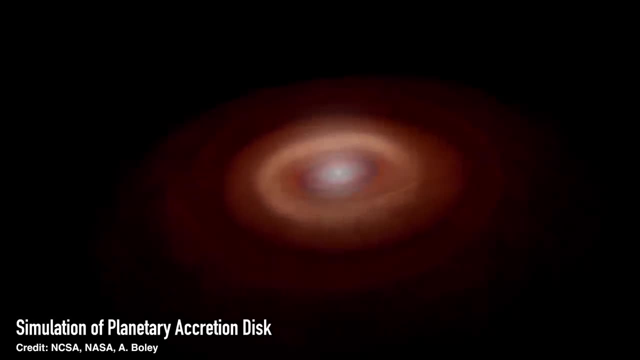 Now I want to chat a little bit about exoplanets now, because there's three studies that have come out related to exoplanets that I want to highlight, Starting with the beginning of planet formation in a dusty disk of gas around a newly formed star, which has been spotted for the first. 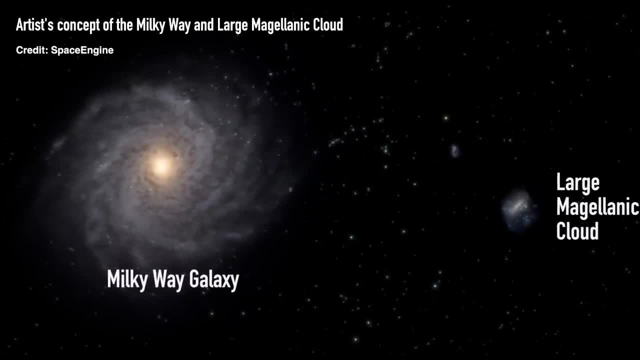 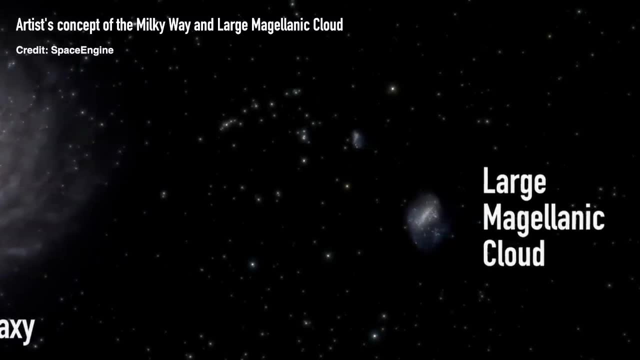 time around a star outside of our galaxy, the Milky Way, in the Large Magellanic Cloud, A dwarf galaxy in orbit around the Milky Way which you can actually spot fairly easily. it's just like a fuzzy blob in southern hemisphere skies when you're away from light pollution. So this research was published. 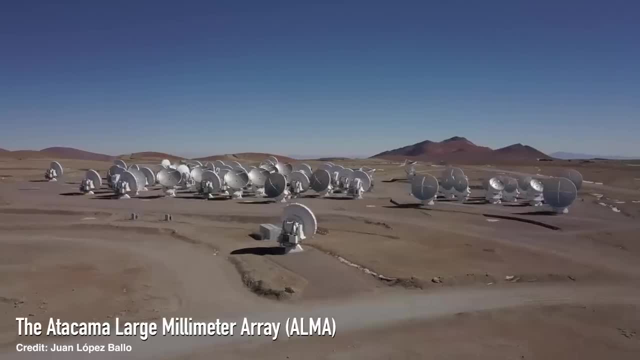 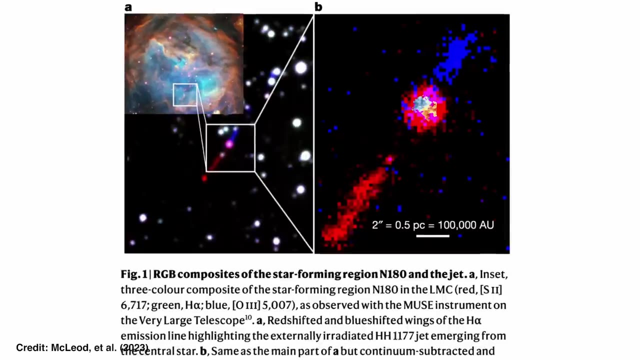 by McLeod and collaborators, who used the Atacama and the Hubble Space Telescope to study the Atacama Large Millimeter Array, or ALMA for short, which is an array of 66 radio telescopes in the desert in Chile to observe a massive young star Similar to those that we see forming in the Milky. 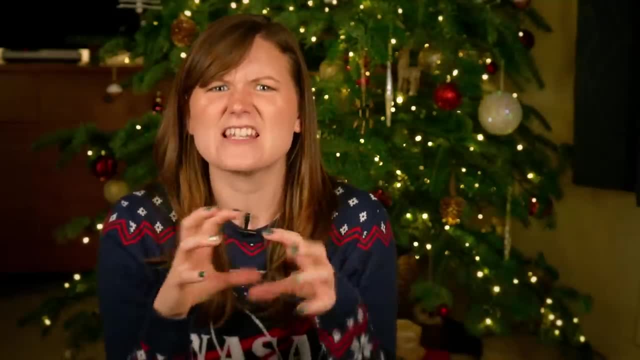 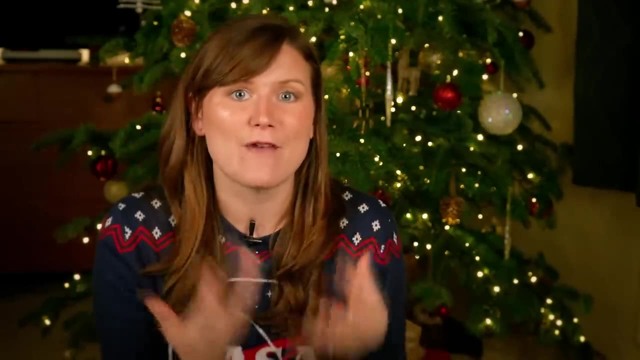 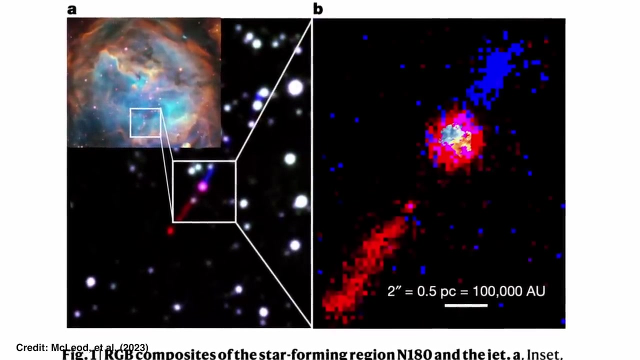 Way you know, these proto stars that have these very thick dusty gas discs around them that are really the beginning stages of planet formation. around that very young star, The star they observed actually has a jet of material being ejected from its poles as well meaning it really is in the very 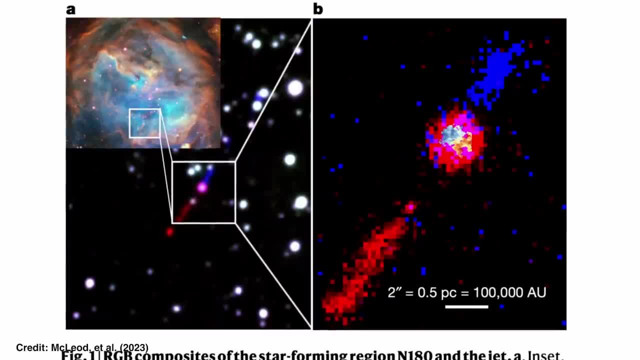 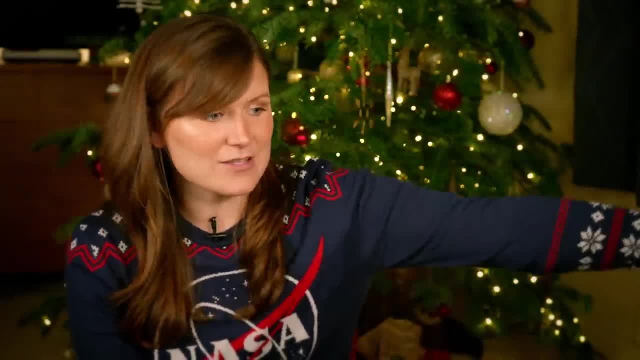 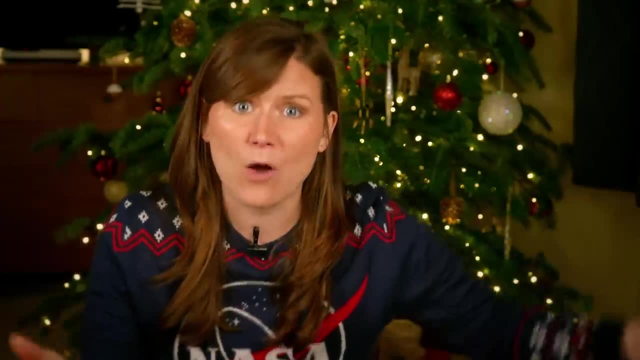 active stages of still forming stuff really hasn't settled down yet Now. the bigger the telescope, the smaller. the thing is that you can actually see in the sky, and ALMA combines all of those individual dishes to make one big telescope that's effectively 16 kilometers wide, so it can see. 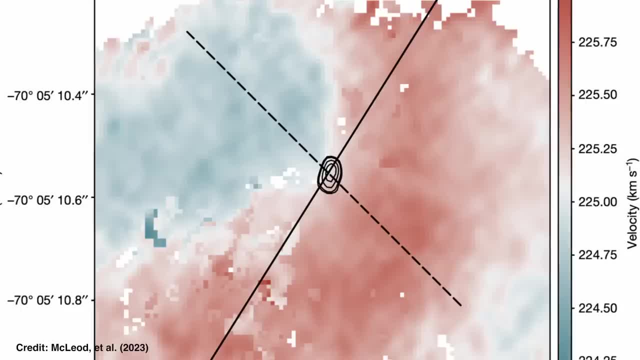 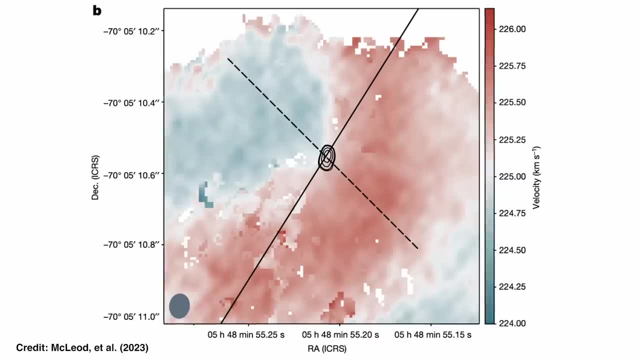 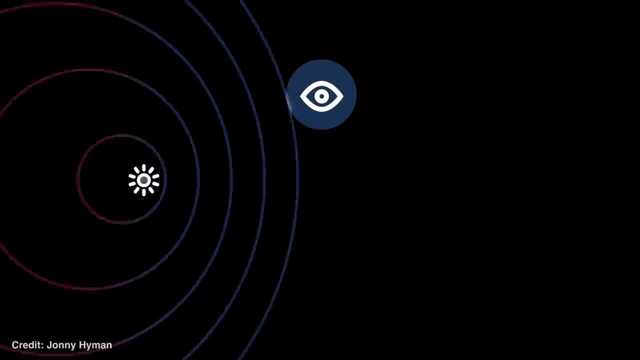 a lot of detail. Thanks to that resolution, they've been able to detect how the gas around the star is rotating. So by focusing on light giving out a very specific wavelength from the molecule carbon monoxide or CO, we can work out if that light has been doppler shifted to longer or 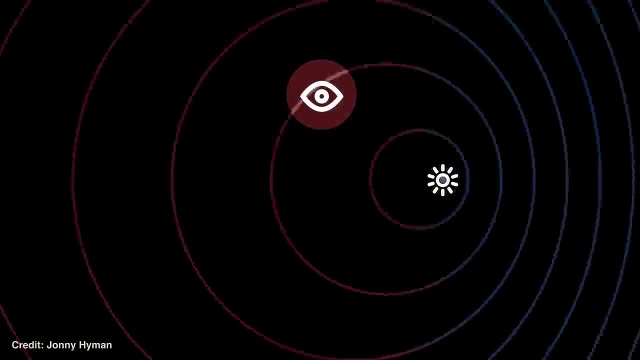 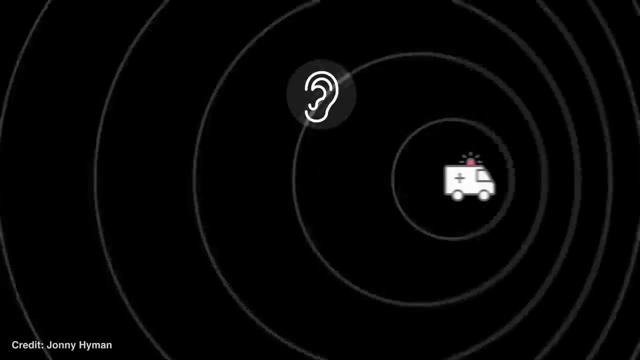 shorter wavelengths because it's moving either away or towards us at a certain speed. Just like with an ambulance, the siren sound wave gets squashed to a shorter wavelength as it comes towards you and then stretched out to a longer wavelength as it moves away from you. So here, 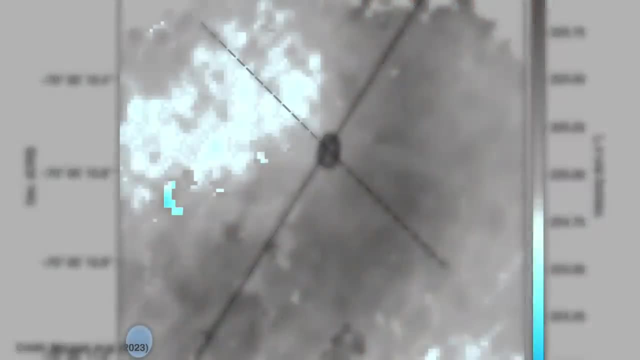 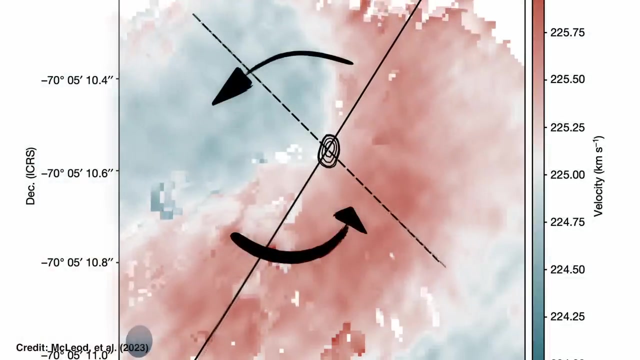 is that data for this star, with material coming towards us colored blue and material moving away from us colored red, And you can see how that rotation of gas has been moving around the star Picked out really nicely. So this is carbon and oxygen containing gas that's orbiting around a. 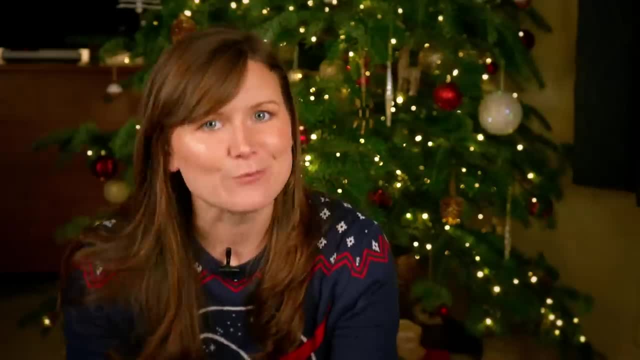 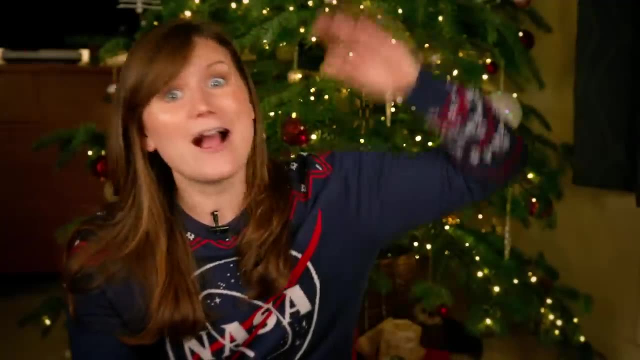 brand newly formed star that should eventually make some planets. So we're really seeing the very beginning stages of star and planet formation and for the first time in a galaxy outside of the milky way. And what's really fun is that you can actually compare the properties of this massive 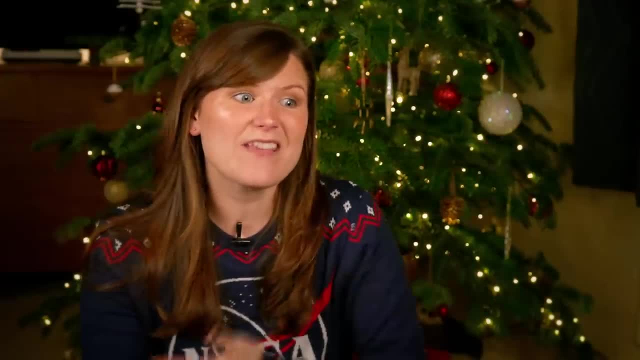 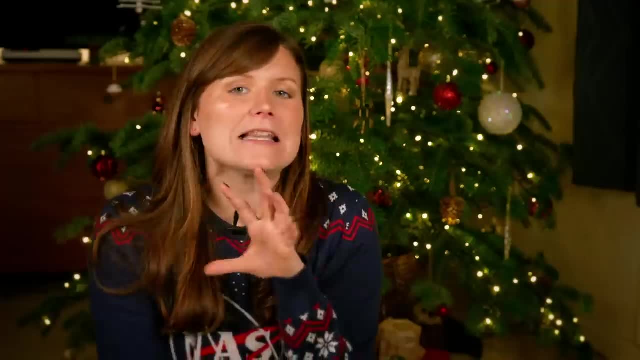 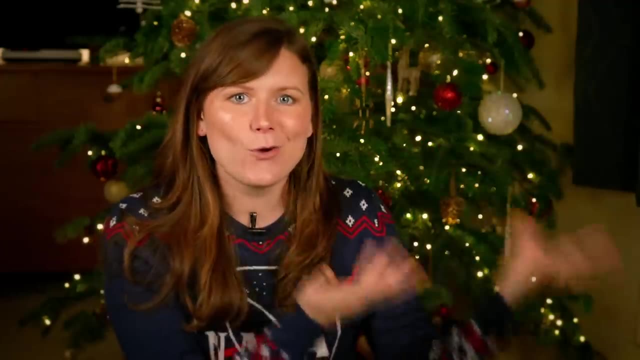 Except for the fact that in the Milky Way they tend to be completely shrouded by dust which blocks our view, so we can't really see what's going on, whereas here there's not really any dust at all. So that tells us a lot about the different sort of like formation conditions in the Milky Way. 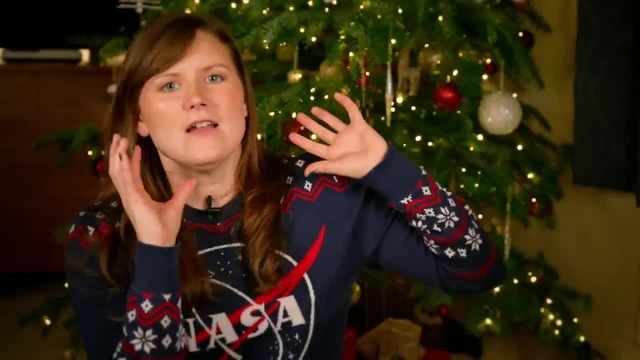 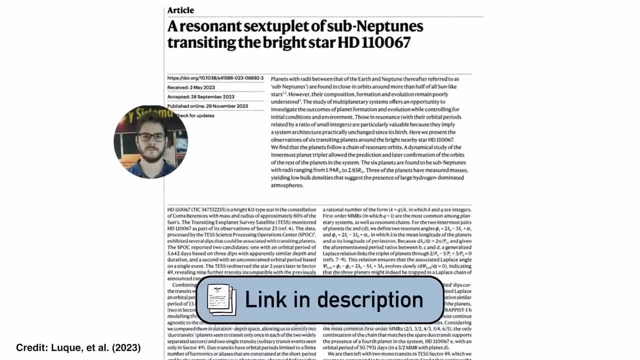 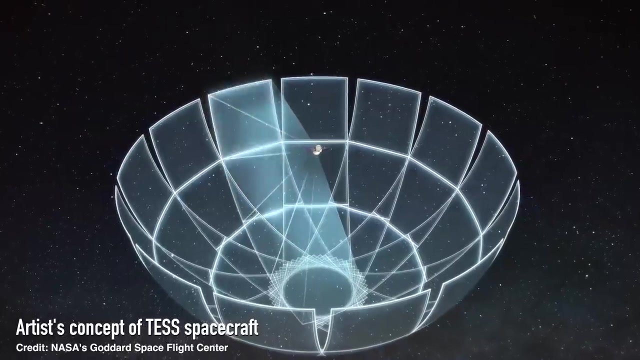 and in the Large Magellanic Cloud. All right, so from very beginnings of planet formation stages to a perfectly formed system of six planets that's been discovered and published by Luque and collaborators. This was found in the TESS dataset, the Transiting Exoplanet Survey. 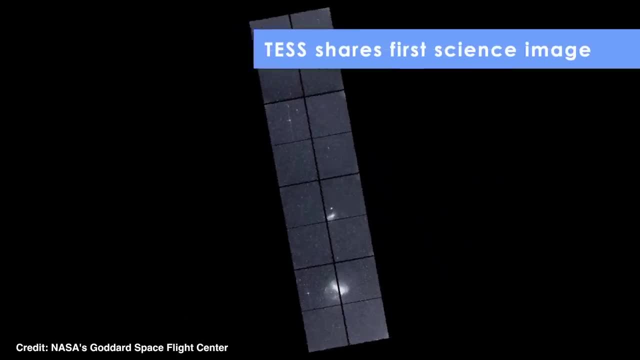 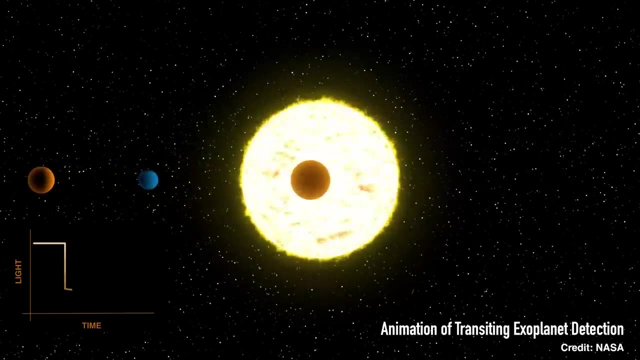 Satellite, A telescope which is in orbit around Earth and is monitoring the brightness of stars in the hope of detecting when a planet in orbit around them passes in front of the star, causing a dip in the star's brightness. This is known as the transit method of detecting exoplanets, because 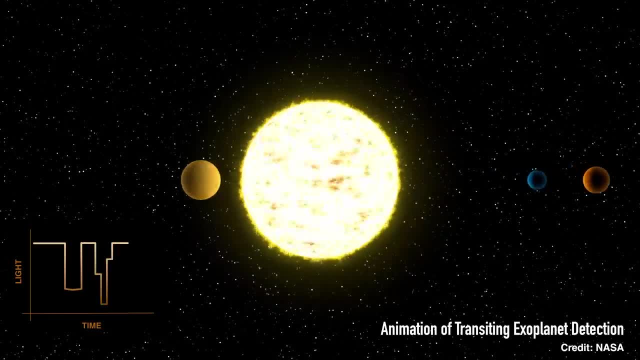 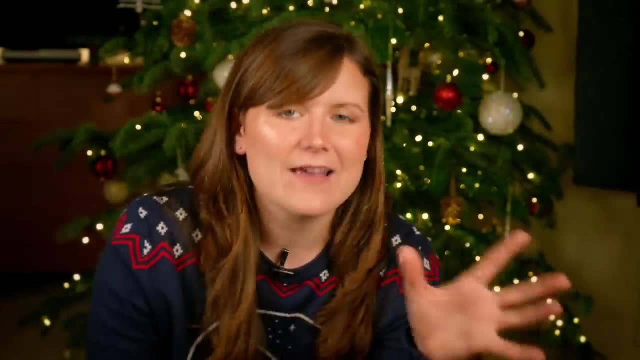 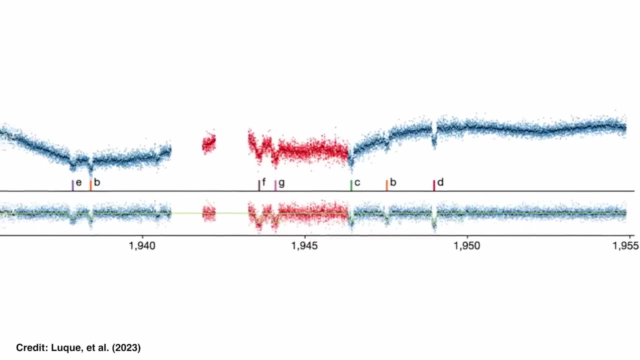 the exoplanet transits in front of its star. Now, the star they were looking at, HD 110067, is around about 80 percent of the size and mass of the sun, and it's been monitored by TESS before, back in March to April of 2020.. That data was processed by the telescope's data pipeline and the algorithm flagged 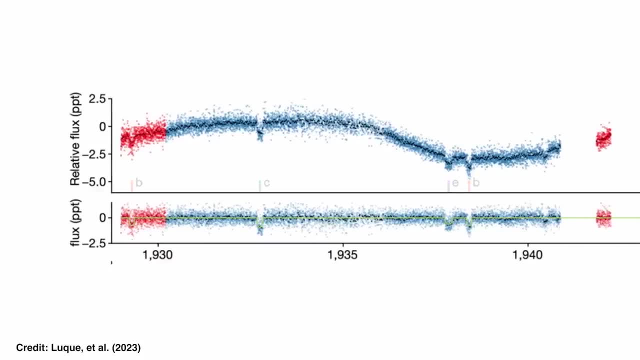 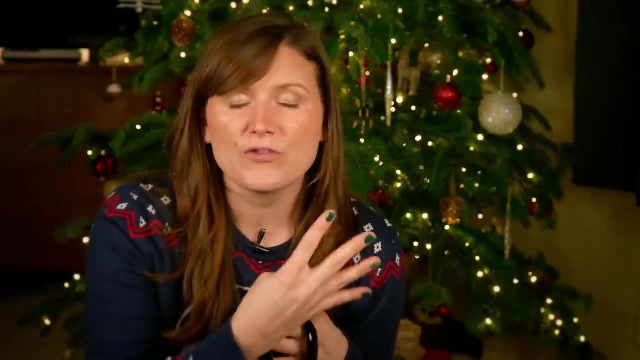 two possible planets based on the transits that it spotted, showing four dips in the brightness. Now it was thought that three of those dips in brightness were caused by one planet and that the fourth dip in brightness was caused by another planet in orbit around that star. But then TESS monitored HD. 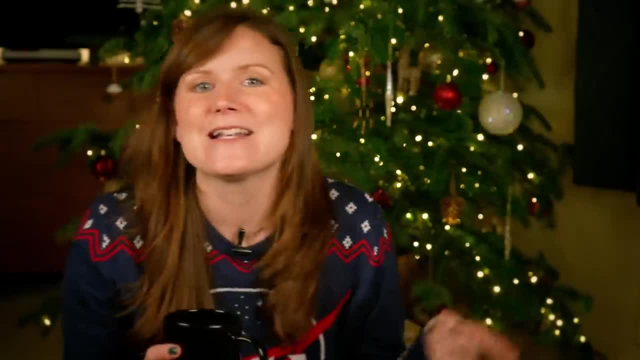 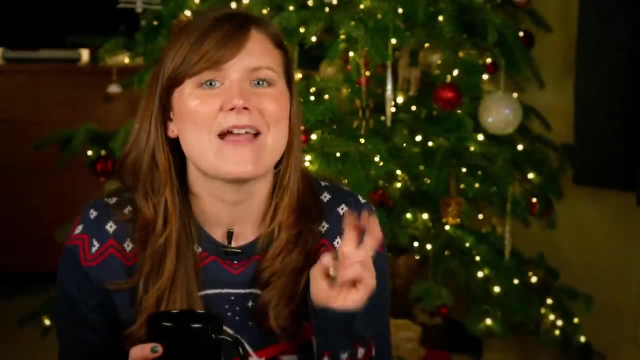 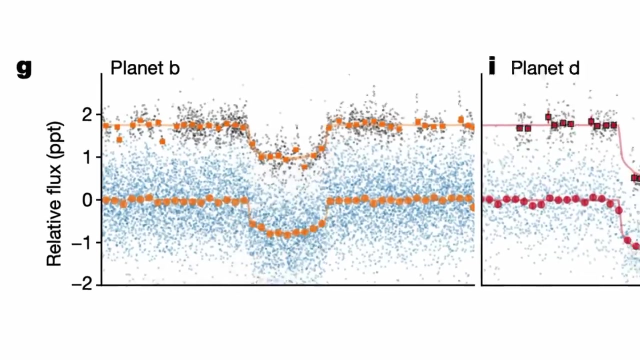 110067, again this time between February and March 2022, and saw nine dips in the brightness of the star which could not be explained by a two planet model. Now, Luque and collaborators first of all noticed that some of the dips corresponded to the same planet, as they had the same shape and blocked the 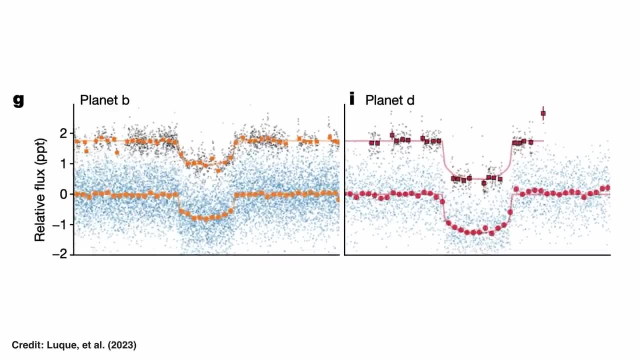 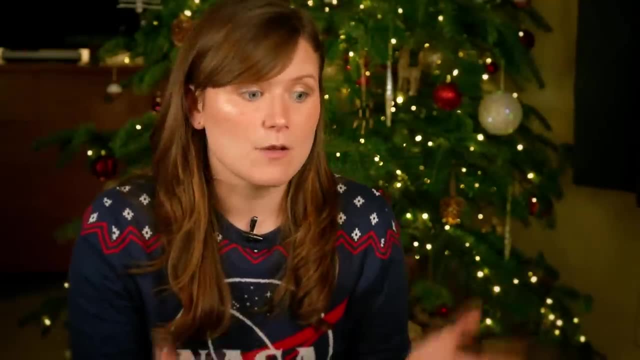 same amount of light That confirmed there was at least three planets in the system. From that data they could then start to make a model of the exoplanet system as they understood it. then, with three planets, You know, you can work out how far away each planet is orbiting from its star and how long. 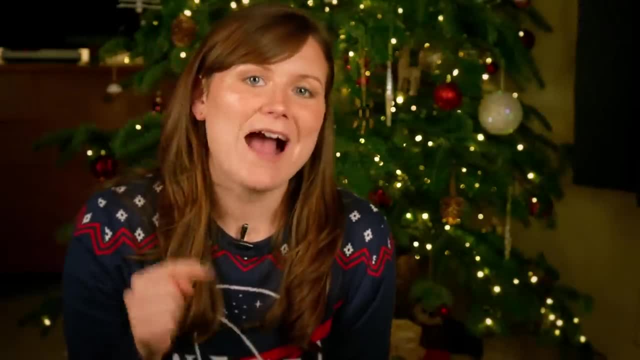 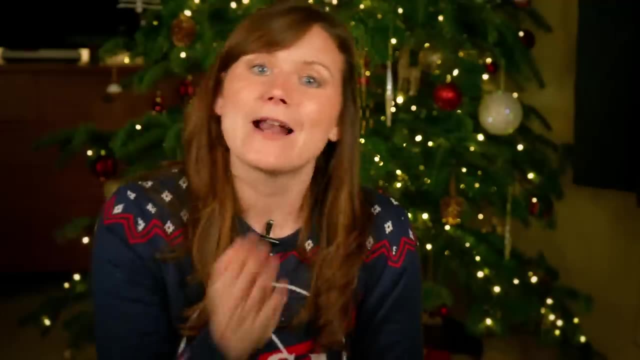 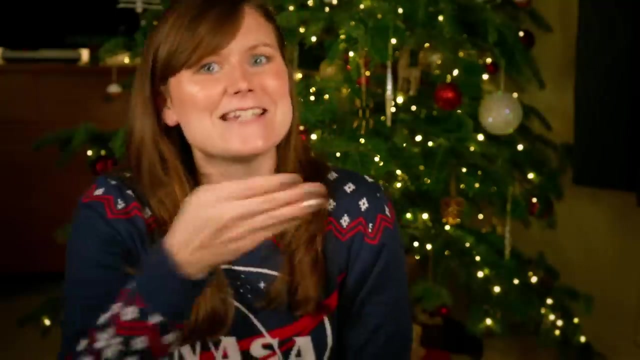 each orbit takes And they noticed that the planets were actually in resonance with each other, a three to two resonance. So for every three orbits that planet B, furthest into the star, makes, planet C makes two orbits. and then for every three orbits that C makes, D makes two orbits. And they 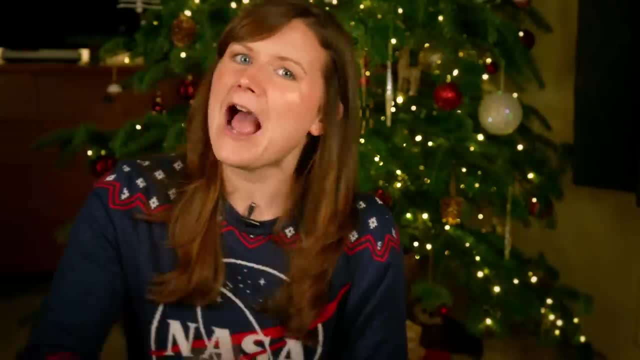 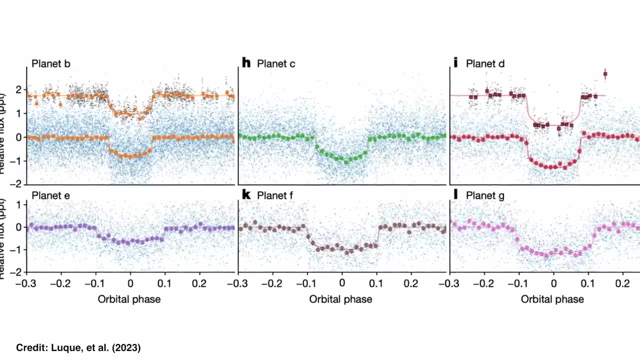 started to wonder: well, if there's more planets in this system, could you carry on this chain of resonance? So Luque and collaborators think the most likely explanation for their data is a six planet system in these resonances with each other, And I love that. one of the best ways to represent 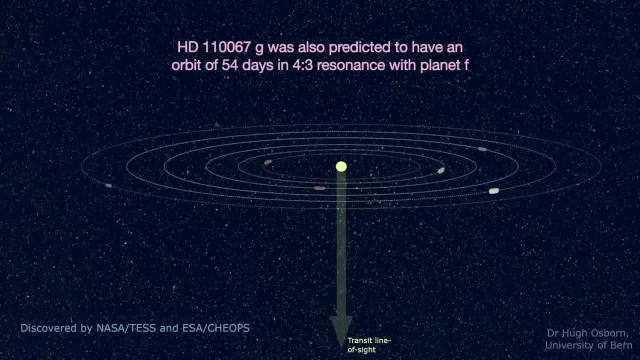 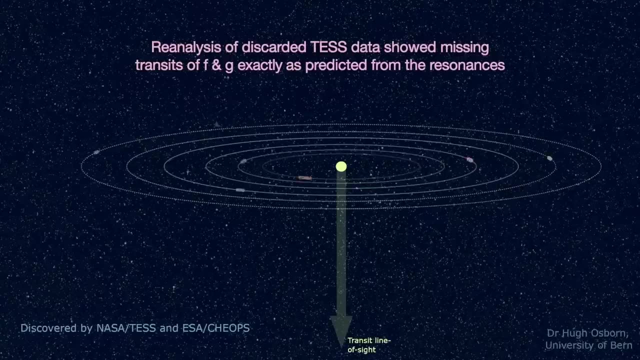 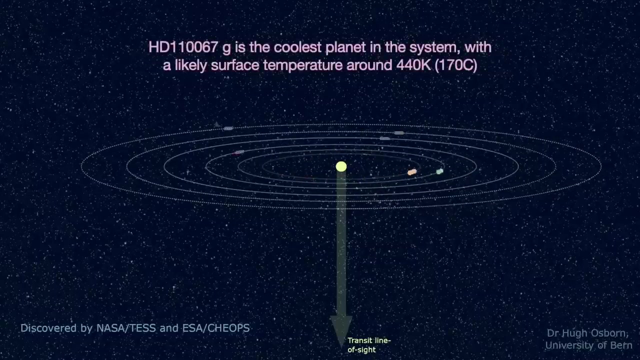 this resonance is through sound. If you play a different note for each planet when it comes back to the same point in the orbit, you can really hear how all of them relate to each other as they go around this star. Now it's pretty sad to say that this is a very long story, but it's a really good way to start the story. Now. it's pretty sad to say that this is a very long story, but it's a really good way to start the story Now. it's pretty sad to start the story Now. it's pretty sad to start the story Now. it's pretty sad to start the story. 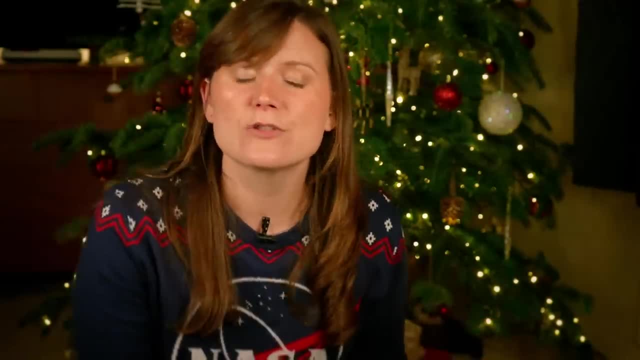 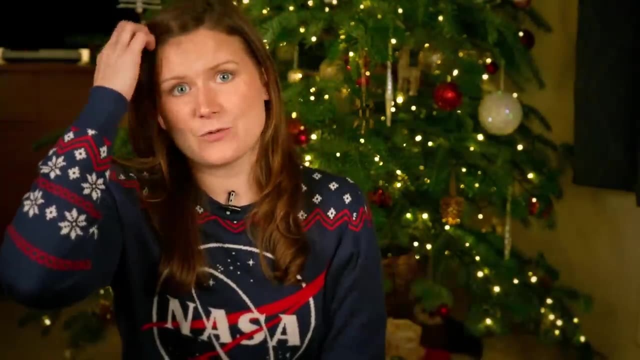 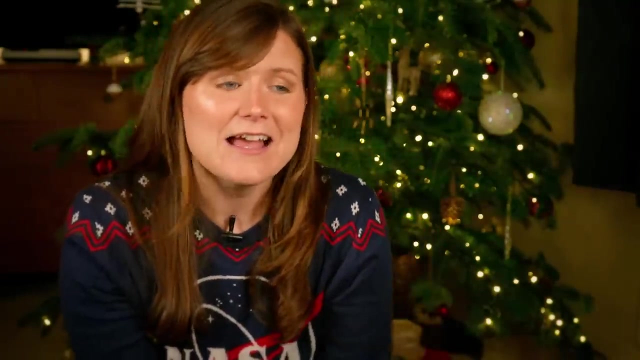 As that is. systems like this are also incredibly scientifically useful, because we think when planets first form around their stars, they start to drift all over the place as they interact with each other, Migrating inwards or migrating outwards, with all those interactions, until they find a place that they're happy In the solar system, for example. we don't think that any of the 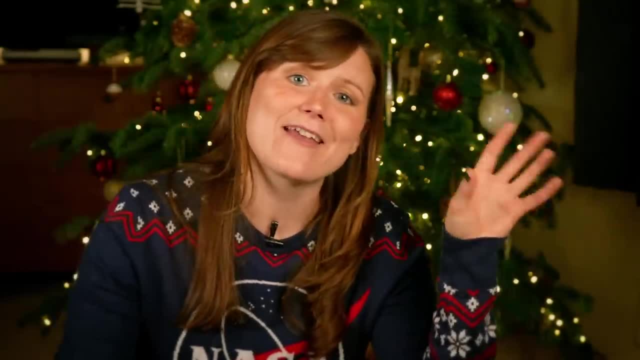 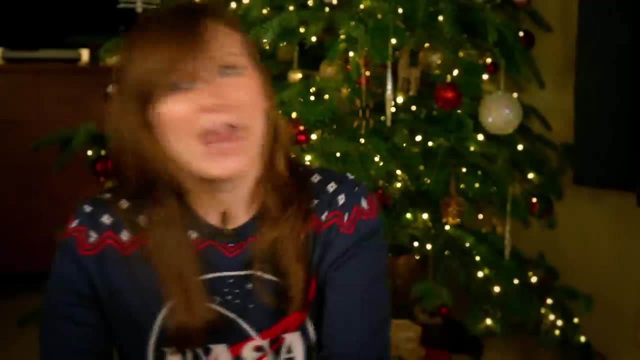 planets are. you know, with their current positions are anywhere near where they actually formed. So this system, HD 110067, to be the first planet in the solar system, to be the first planet in the solar system be in this perfect chain of resonance, has to have formed that way from the beginning, to be like that. which means that the positions they're in now are the positions that they were in when they formed. So we can study. you know, how do the conditions that a planet formed in, like the environment it forms in, then affect like what size the planet is and what it's made out of? So when we look at the 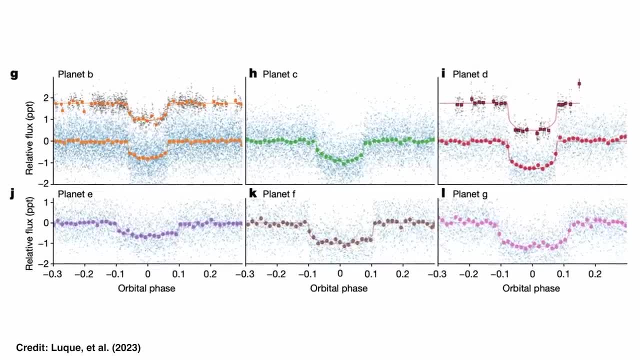 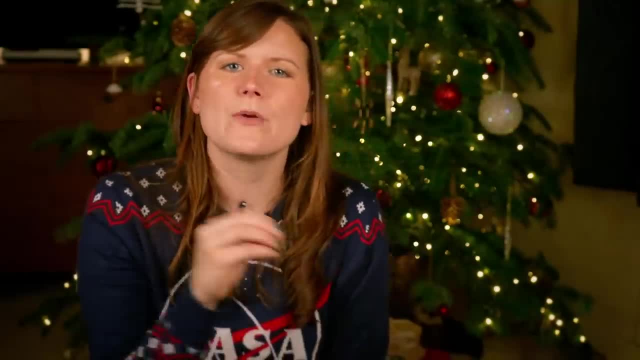 data of each of these transits. here we can actually work out an estimate for their sizes, for how much light they block, and it turns out that these six planets are all what we call sort of super earths or sub-Neptunes, falling in that size gap from around about two to three times the radius of the earth, But given their estimated masses, we think that means they're actually incredibly low density. so it's very likely they have very sort of like thick gas atmospheres. they're much more like Neptune than a rocky planet like earth. On top of that, HD 110067 is the brightest star to have been. 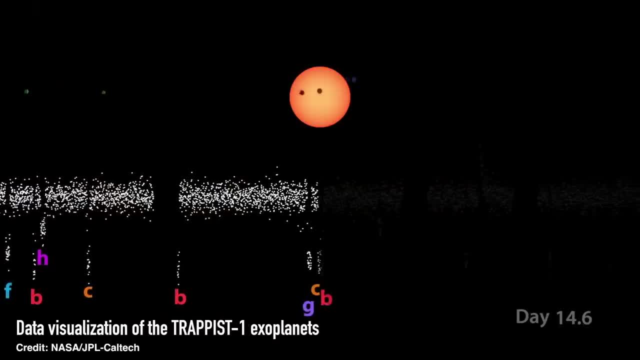 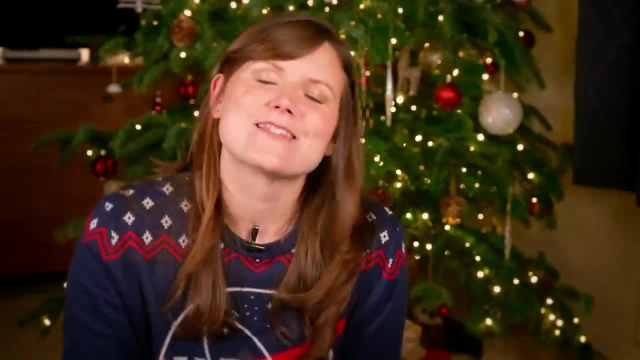 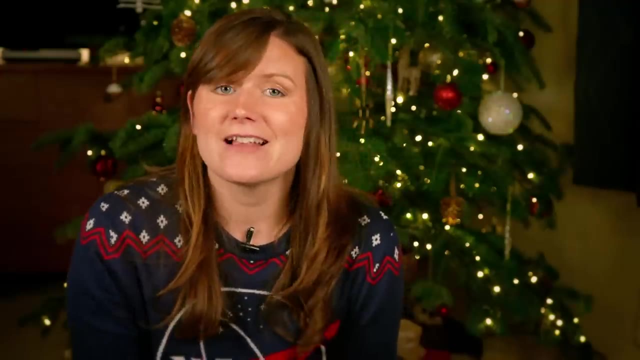 transited in the past. So it's actually very likely that we can then look at more than four transiting exoplanets. So, although we found seven and eight planet systems before, they're around much smaller and cooler stars, Unlike HD 110067, which is much closer in size and mass and temperature to the sun. 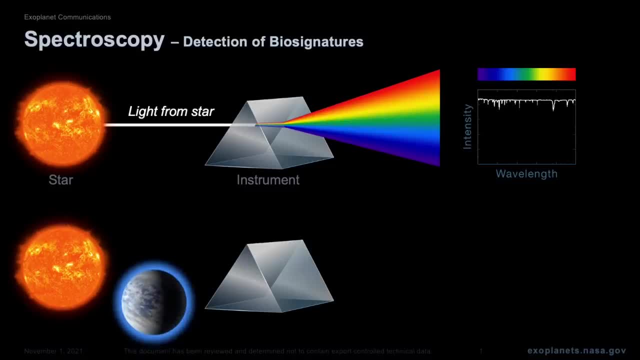 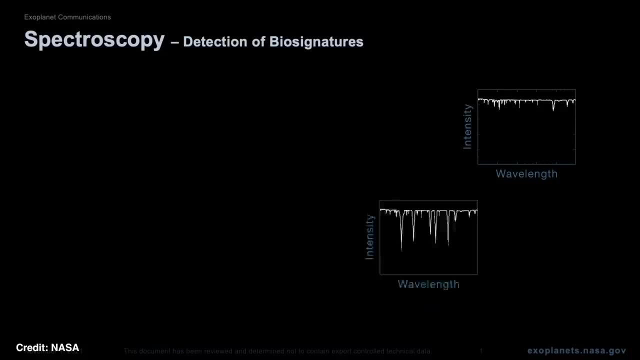 So it's actually very likely that the James Space Telescope is now also going to observe these exoplanets and try to detect the light that passes through the planet's atmosphere when they transit, and then look for the fingerprints that are left behind by certain molecules to work out what their 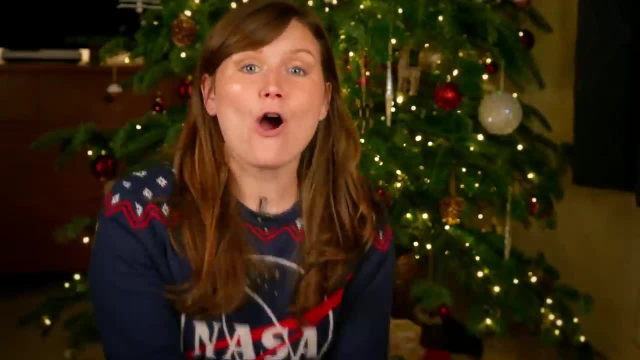 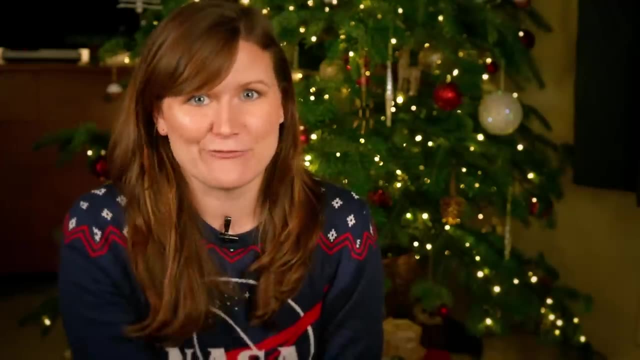 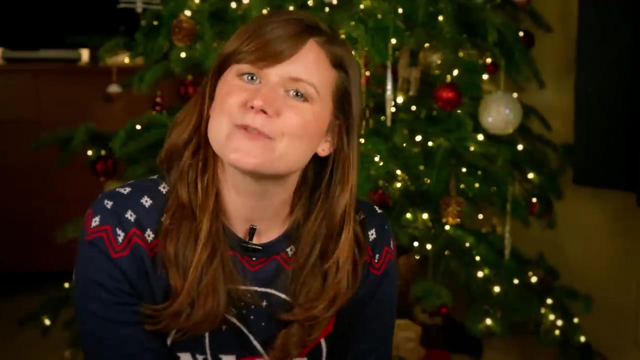 atmospheres are made of, And then again be able to correlate that back to the environment in which these planets formed, because that hasn't changed since they formed. So a very exciting system, one that I think is going to get a lot of attention and be observed a lot in the next couple. 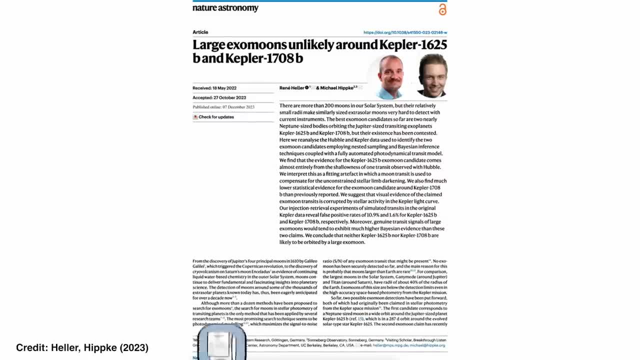 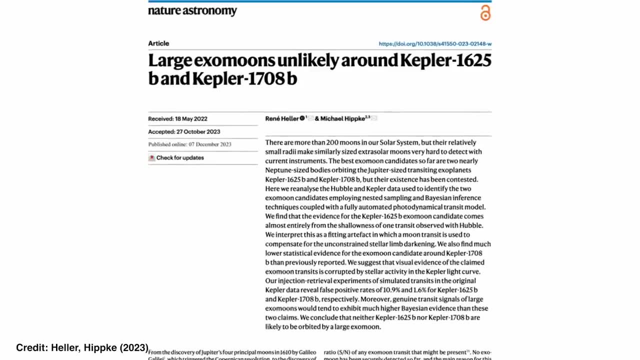 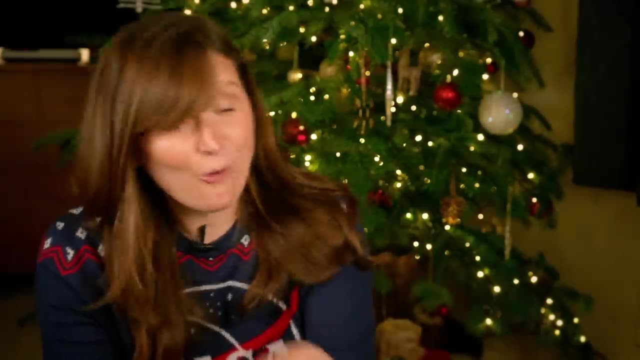 of years. Right now, the last exoplanet research paper I want to talk about is this one by Heller and Hipke, who've made us all very sad this month by saying it's unlikely that we've ever detected any exomoons, ie moons in orbit around planets, in orbit around other stars. Now, there's only ever. 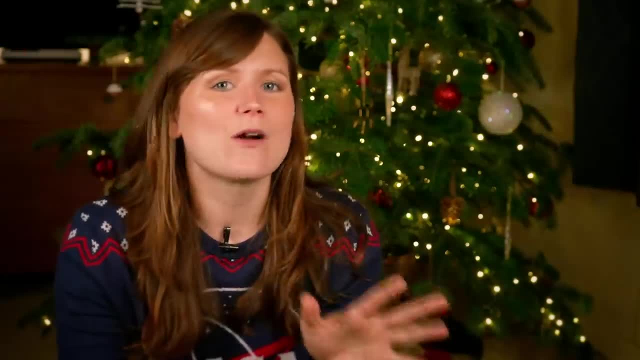 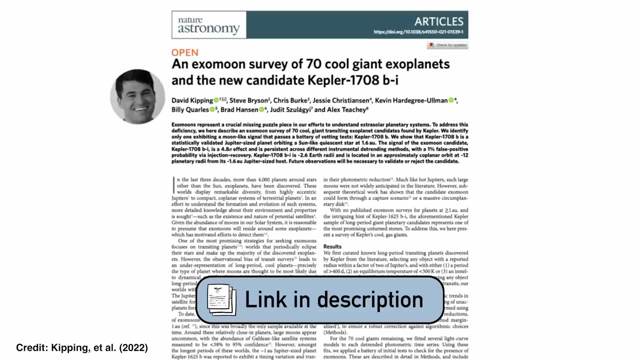 been two planets that anybody's ever claimed to have evidence of an exomoon in orbit around. The first was claimed in 2018 by Tichy, Kipping and Schmidt, And then again, the same group claimed to have found another exomoon by surveying some of the exomoon's, exomoon's, exomoon's, exomoon's, exomoon. 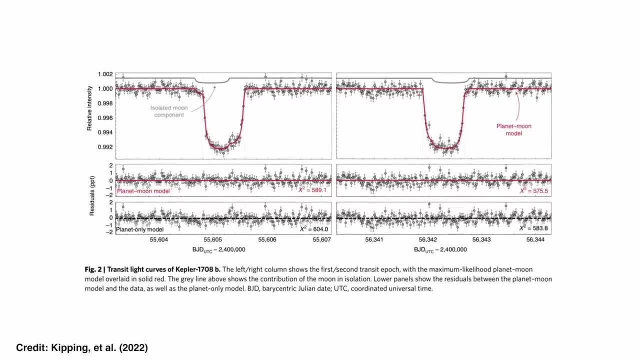 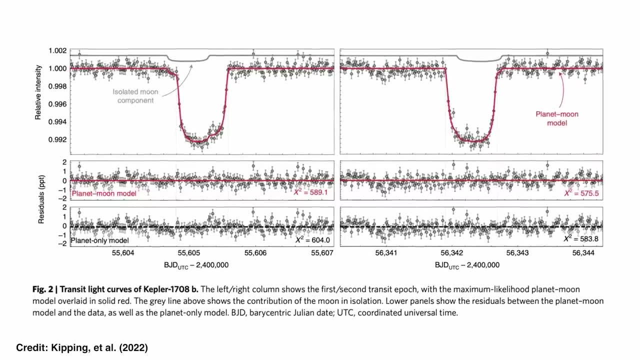 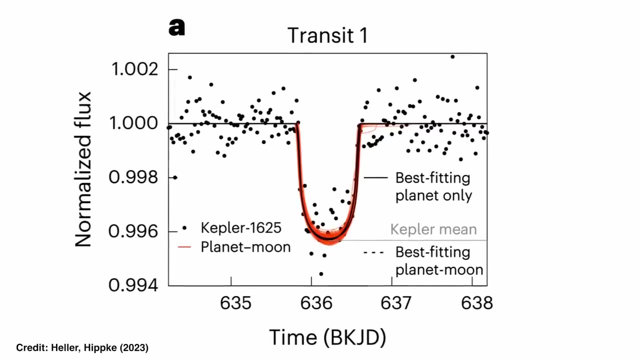 70 exoplanets and looking for those extra dips in brightness that would be caused by the moon blocking light from the star as well as it trails the planet in its orbit. But now Heller and Hipke have re-analyzed that data and said that you can fit those transits just fine with just a planet. 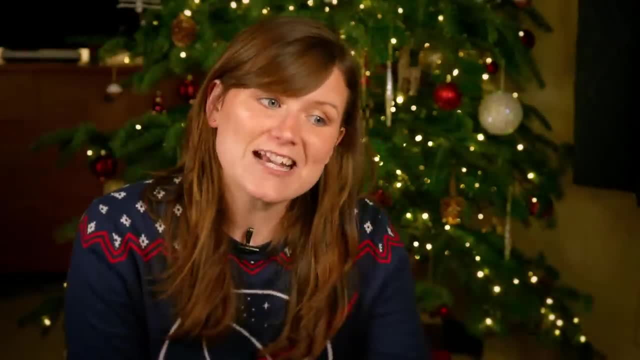 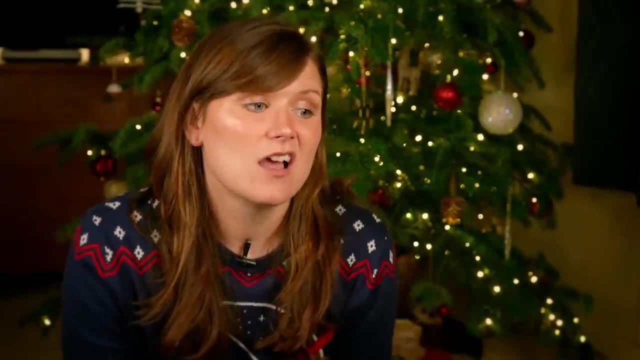 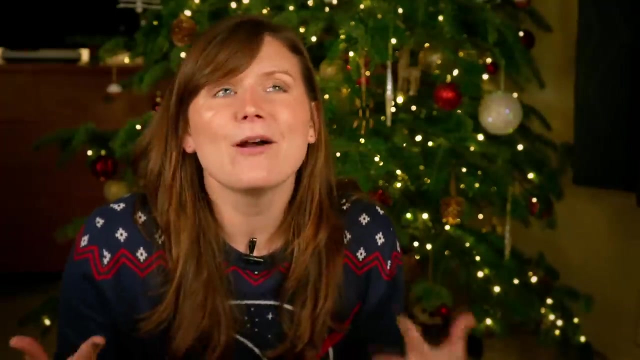 only model And that the signal that the previous groups had claimed was the exomoon was actually just noise in the data, or maybe even just the star dimming weirdly on the edges, Which is kind of sad. but you know, sometimes that's just the way the data crumbles. But if we think about 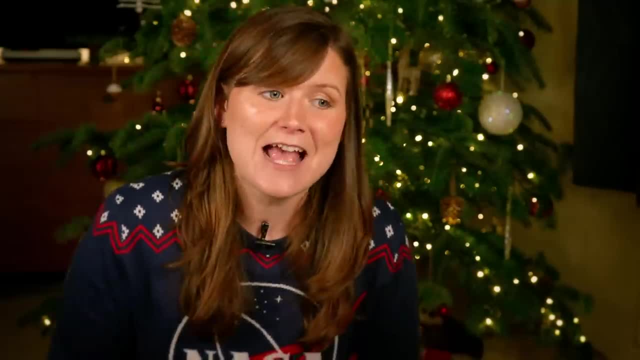 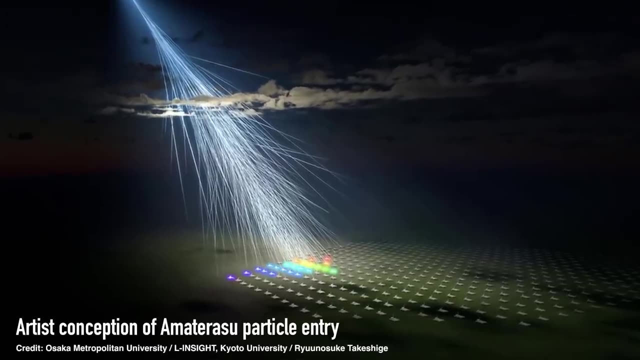 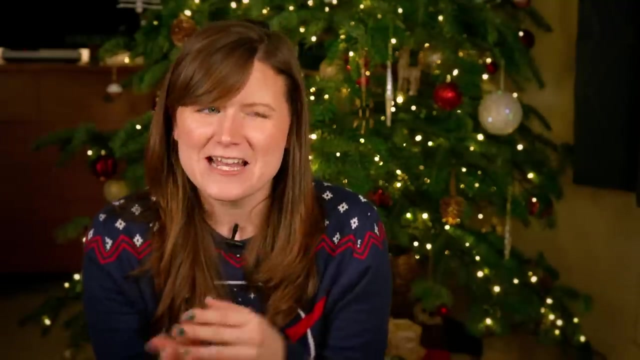 we should be able to find them with our current instruments. It's just knowing where to look. that's the problem. And finally, let's chat about the third highest energy cosmic ray particle to ever have hit the earth's atmosphere since records began. Now it hit back in. 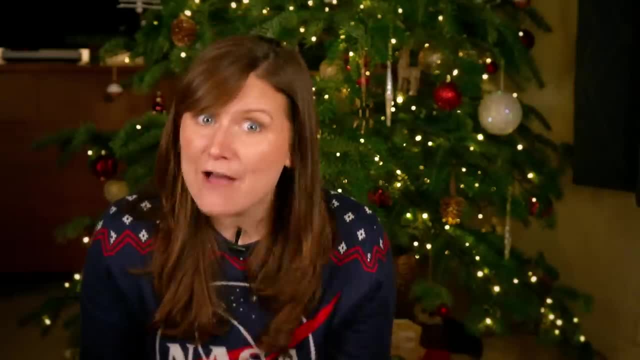 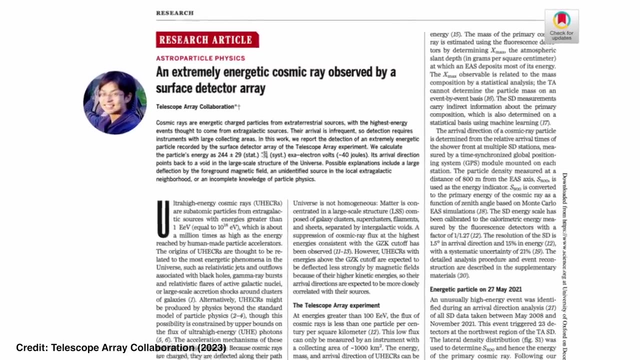 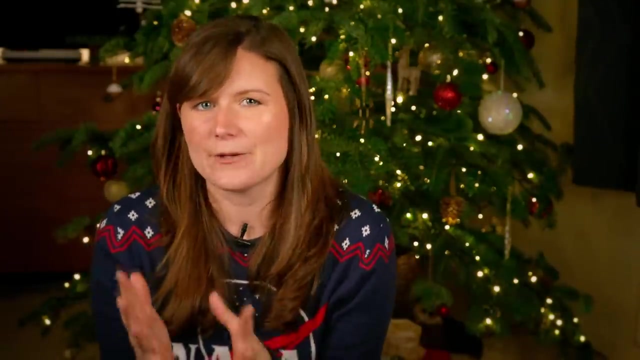 May 2021 and, after a lot of careful analysis, the research has now been published in November 2023 by Fujian Collaborators from the Telescope Array Collaboration. This cosmic ray event has been dubbed Amaterasu, after the sun goddess in Japanese mythology, but it's highly unlikely. 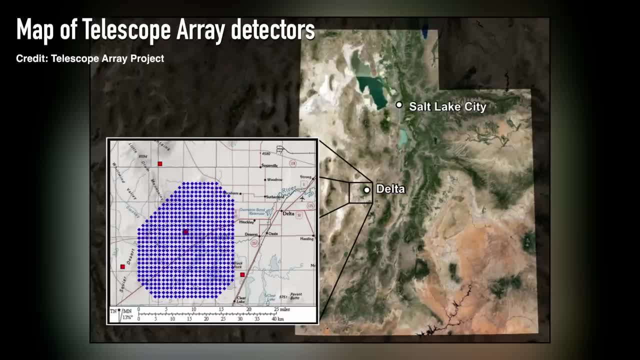 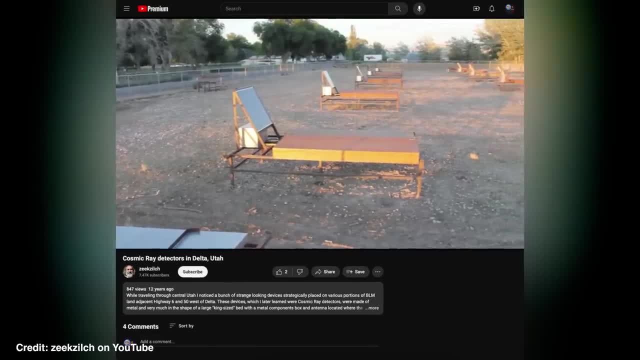 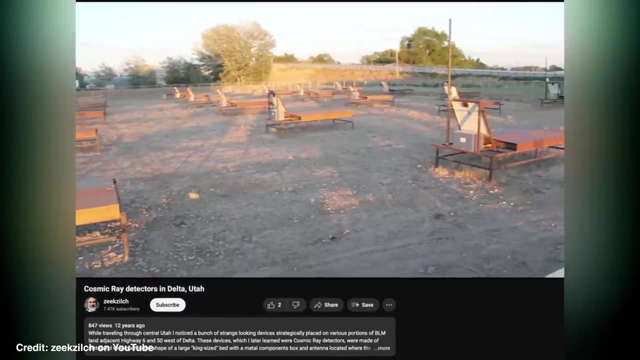 that this event actually has anything to do with the sun. So this was detected by the Telescope Array, which is a cosmic ray detector in Utah in the USA, with an individual detectors of about three meters squared, each arranged in a grid separated by 1.2. 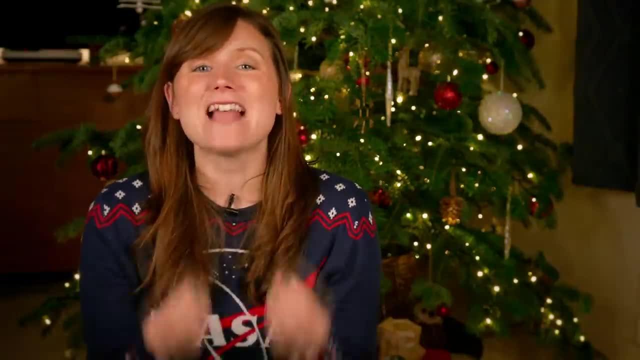 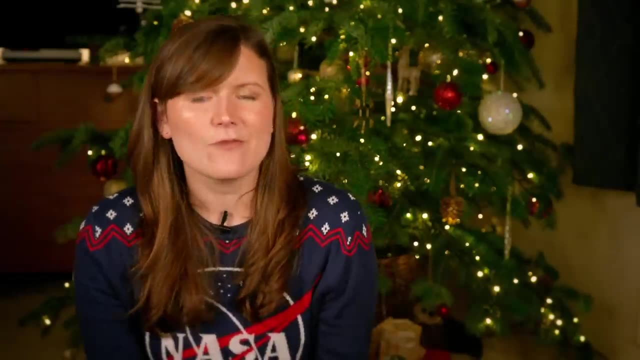 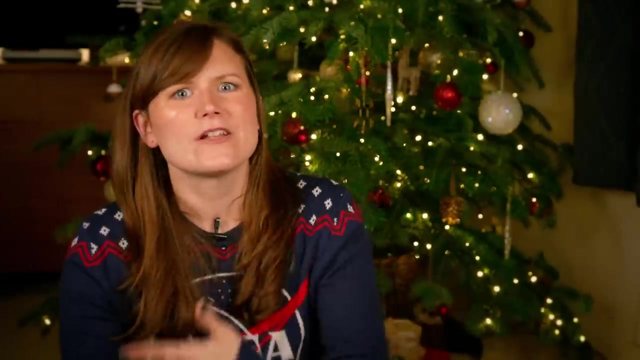 kilometers. It gives the whole array a collecting area of 700 kilometers squared, which is continuously monitoring for these cosmic rays. Now, cosmic rays are single particles, so think like a single proton, so you know, like the nucleus of a hydrogen atom or the nucleus of a much heavier atom, And they're 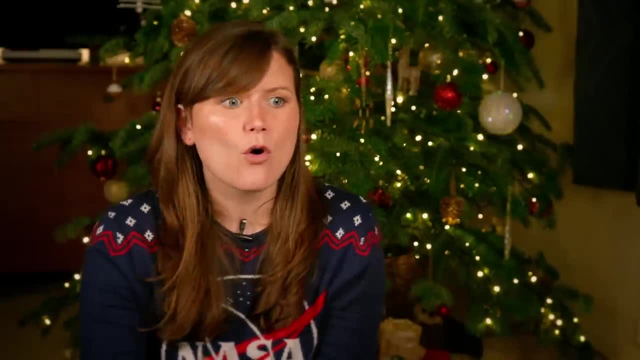 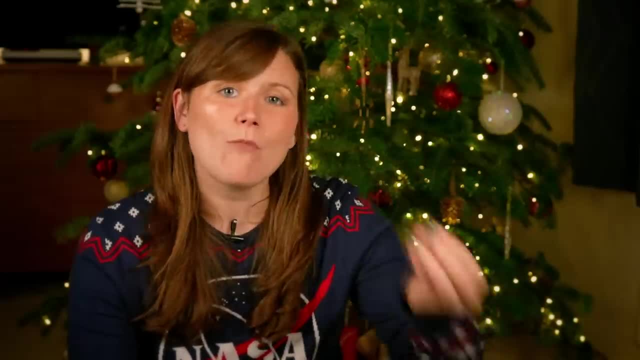 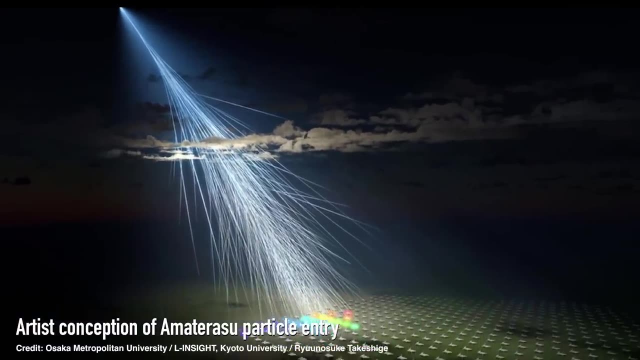 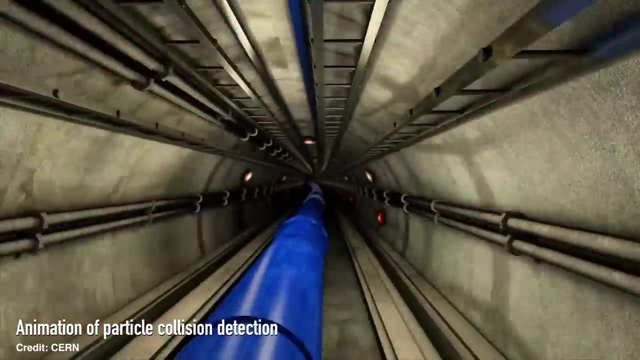 universe before it happens to impact with another molecule at the top of the earth's atmosphere, And the energy in that collision goes into creating a huge shower of other particles, which is what's then detected on the ground by these detectors. This is just like what happens in a particle. 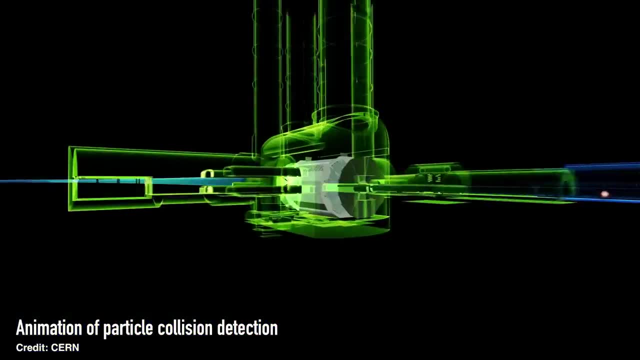 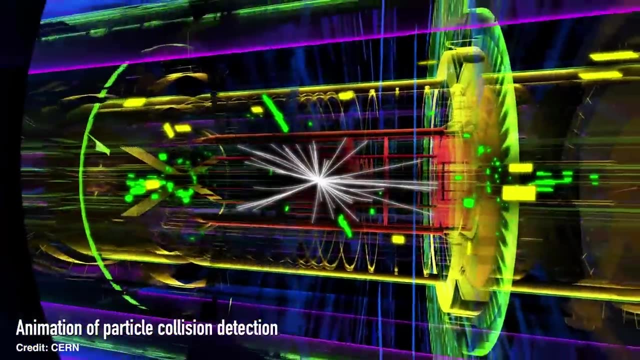 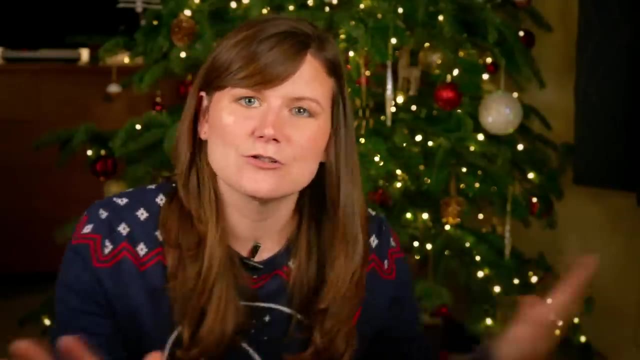 accelerator that particle physicists build here on earth, like in the LHC at CERN, The particles are accelerated to huge speeds, collided together, and then we observe the particles that are created in the high energy of the collision. Now I was physically first to think of, like you know, the energy generated in these big particle coliders. 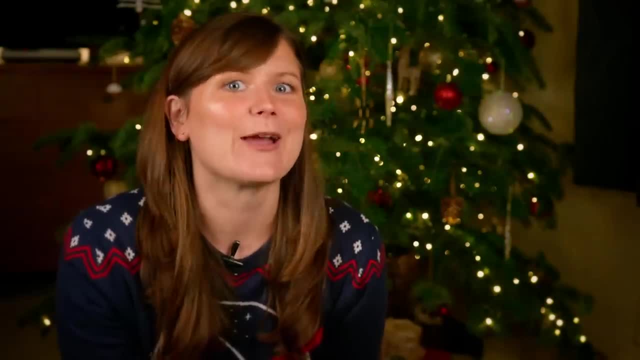 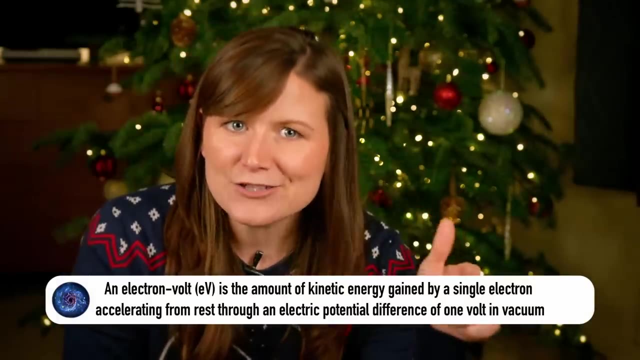 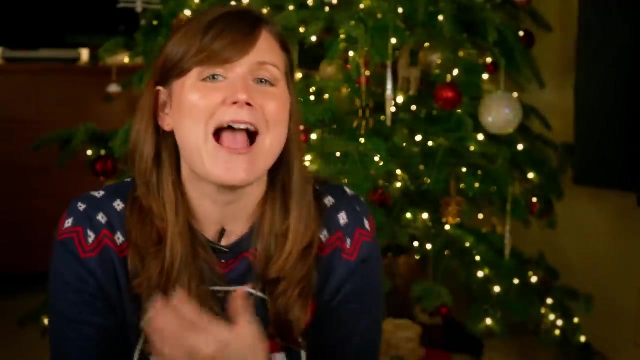 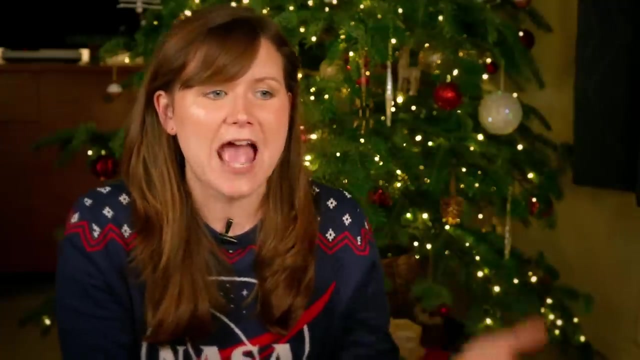 that particle physicists build as being like pretty big right, like the maximum that we've achieved is roundabout Seven teriggs electron volts. the amateur ASU offical had an report 14 million times higher than that, at 240 times exa electron volts, like it's just huge. i mean the reason we use electron volts, usually for the 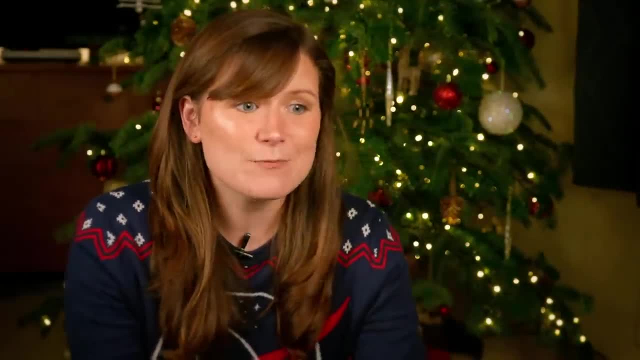 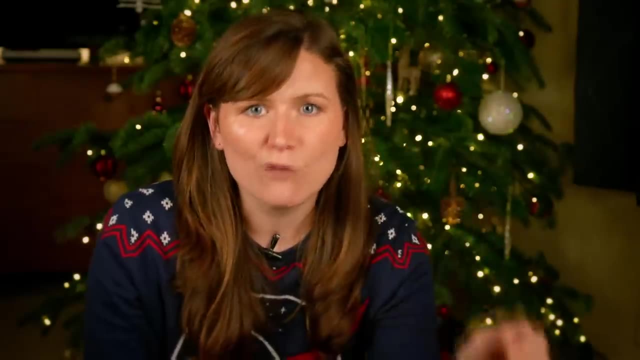 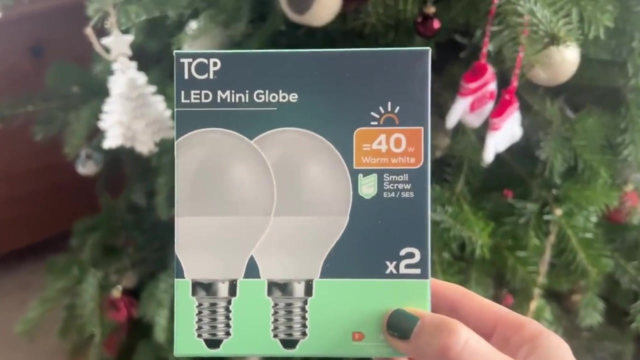 energies of just like these single subatomic particles is because they are so much smaller than the everyday energies that we're used to dealing with. but 244 exa electron volts is 39 joules. so if you've got a 40 watt light bulb then that's 40 joules of energy per second. that it's. 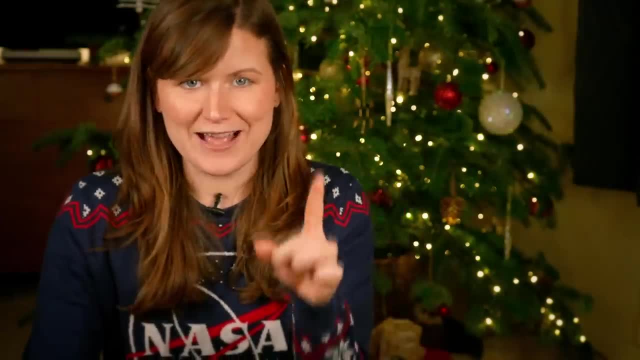 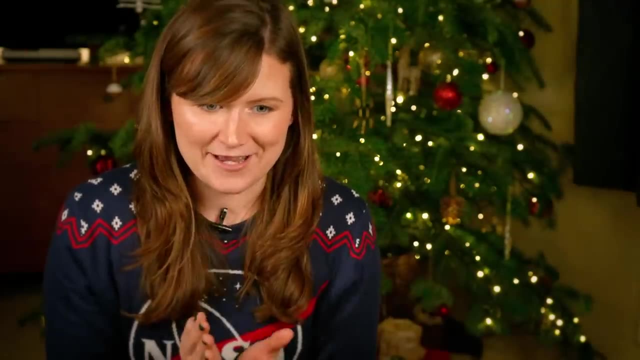 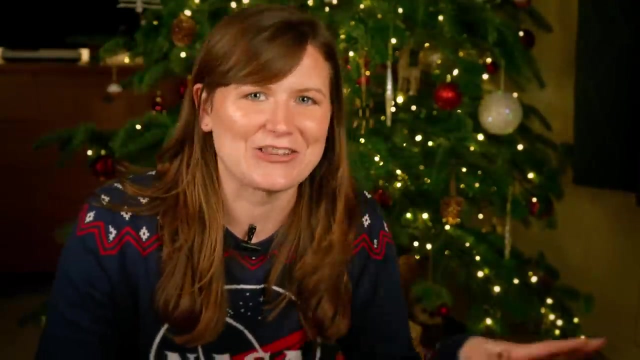 using to stay lit. so one tiny particle hit the top of the earth's atmosphere with the same energy that an entire light bulb uses in the space of a second. i've also seen someone calculate it as the same energy of a brick dropped from waist height to the ground. like that kind of. 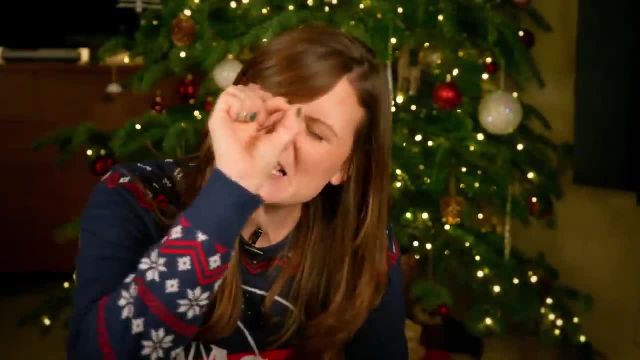 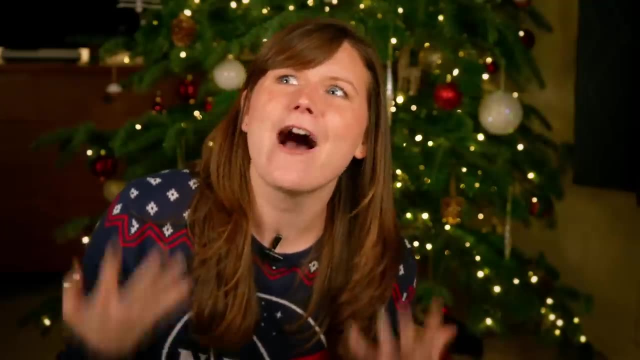 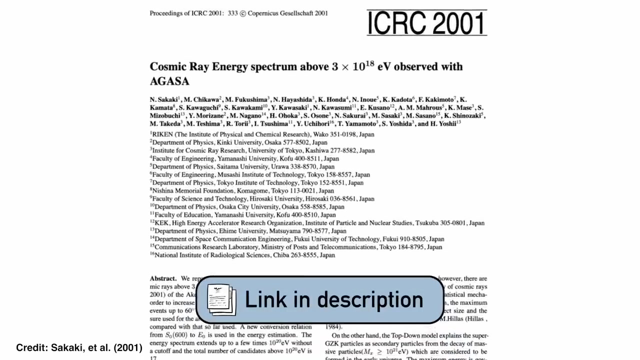 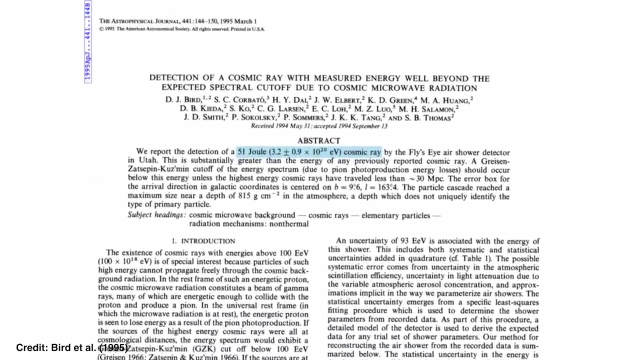 concentration of energy in one single particle is absolutely incredible, and yet it's still non-existent. not the highest energy cosmic ray particle that we've ever detected. In 2001, a 280 exer electron volt cosmic ray was detected and in 1991 there was a 320 exer electron volt cosmic ray detected. 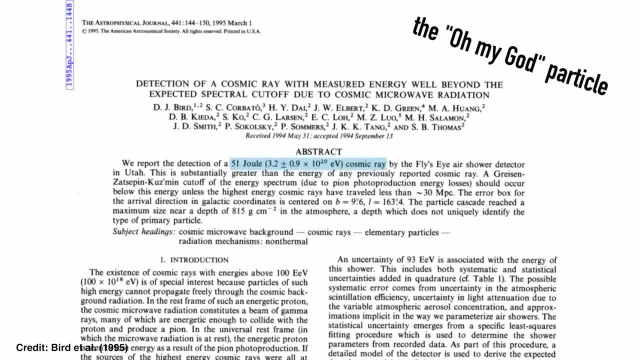 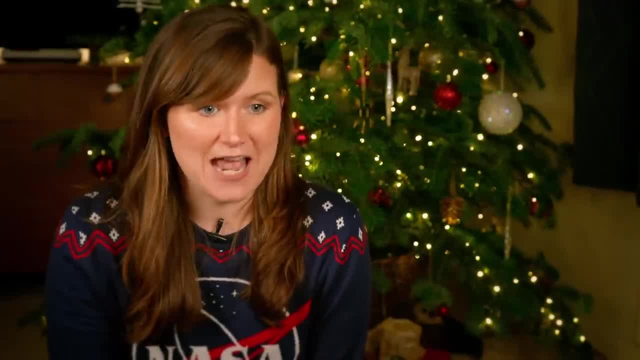 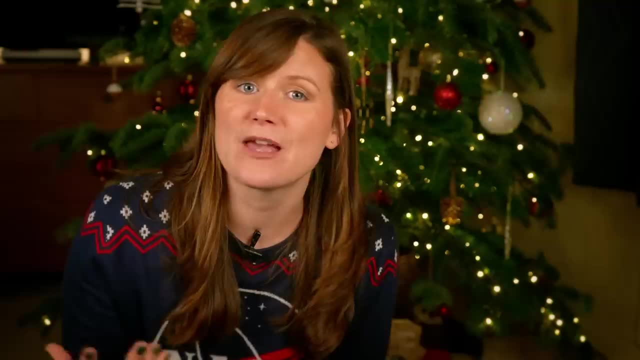 dubbed the oh my god particle because it was so energetic. That makes the Amaterasu particle the third highest energy cosmic ray we have ever detected, at 813 billion times more energetic than a typical cosmic ray that you would detect. Question is: what caused it? Well, here you can see. 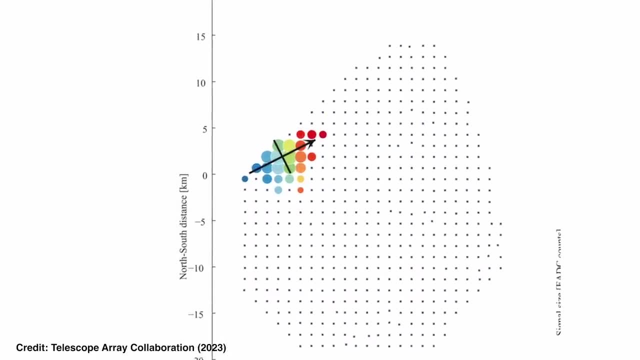 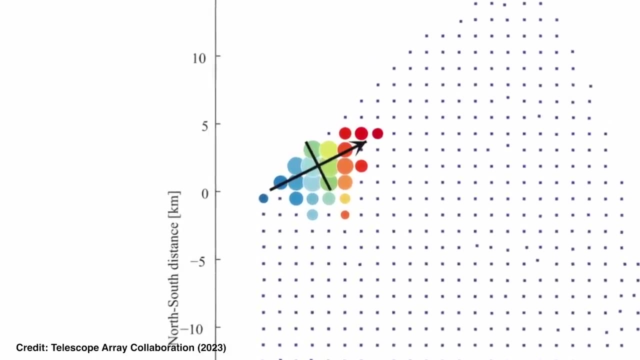 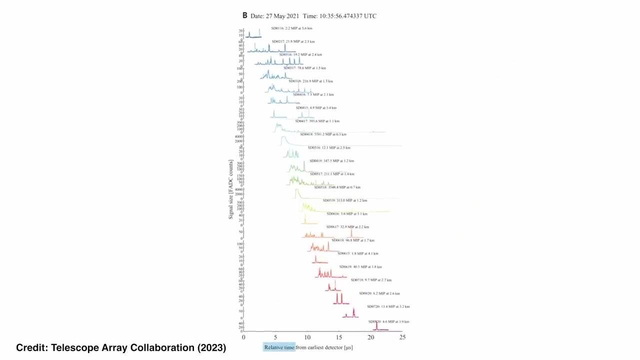 which detectors in the telescope array actually registered the particles from the shower of particles that was generated when the cosmic ray hit the top of the atmosphere, and the color here corresponds to the time that the detector was detected. So the color here corresponds to the were made with just microseconds separating the signals on the different detectors. It's really. 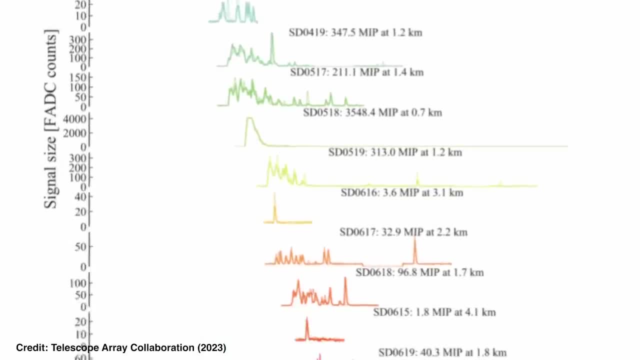 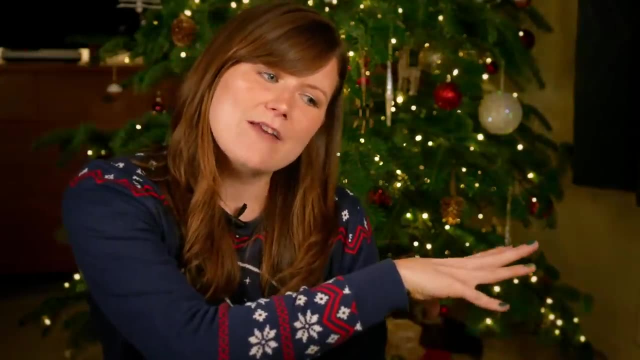 clear. if you plot the data like this, showing what the signals look like at each detector against the time that they were detected on the x-axis. Now, from this delay, and when all the signals arrived, you can use it to sort of triangulate back again to work out the direction. 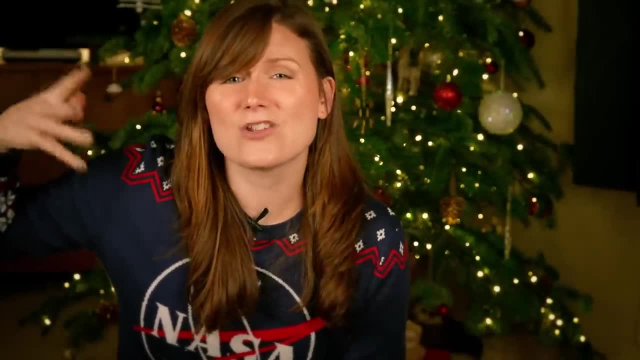 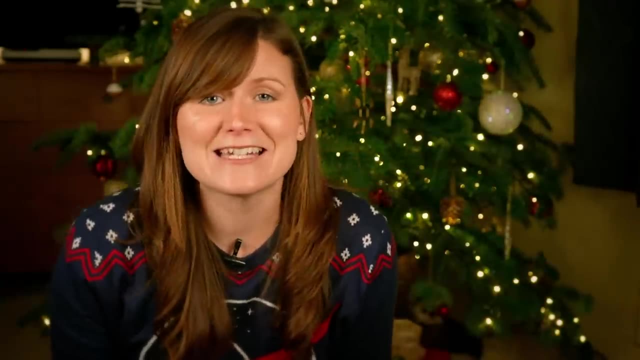 in the sky that the particle has come from. Obviously it's not perfect, because as soon as the particle hits, the shower then spreads out over a wide area, But it gives you a rough idea and at least allows you to narrow it down to about half of the sky at. 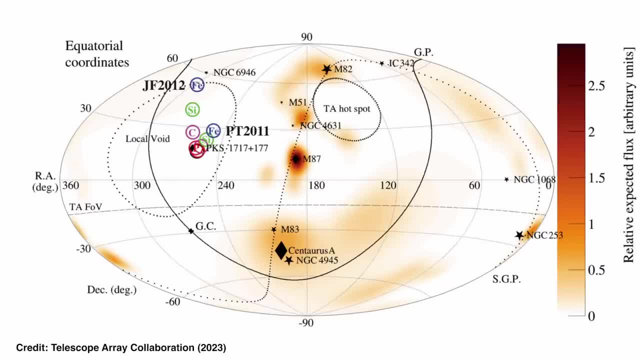 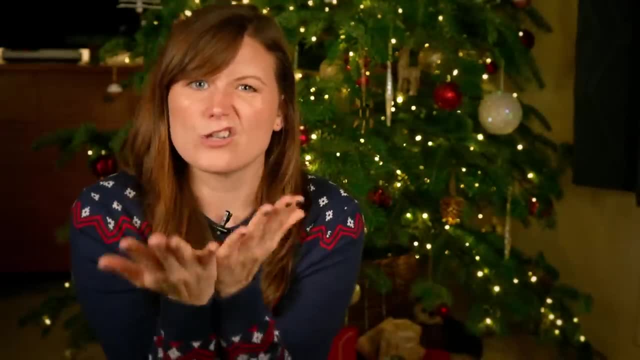 least That's what this diagram shows here. This is the whole sky mapped out and flattened onto the page. That's why it's sort of like egg-shaped, because you've taken like the inside of a sphere and then like flattened it out onto a page. But the black solid circle here is the region which 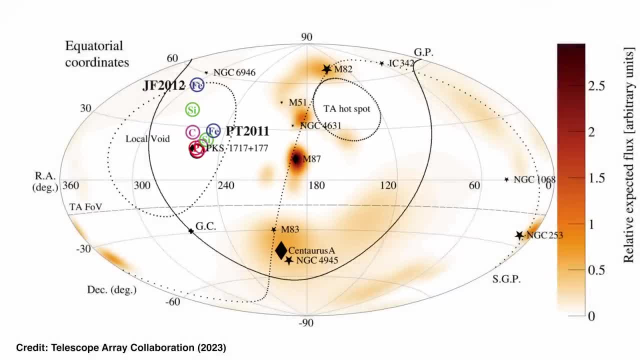 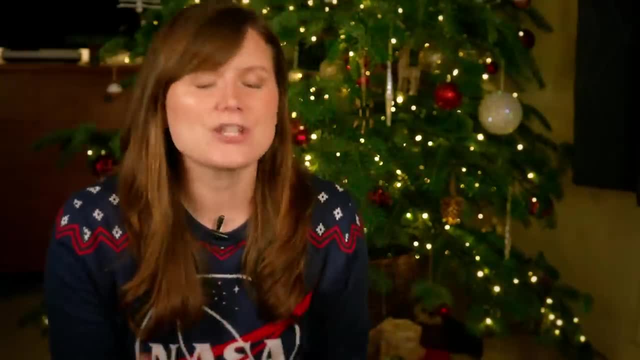 the Amaterasu particle could have come from. So I'm sure you'll agree it's pretty huge. Now you can look within that region for known objects that give out very high energy radiation: high energy particles, Things like supernova or galaxies with supermassive black. 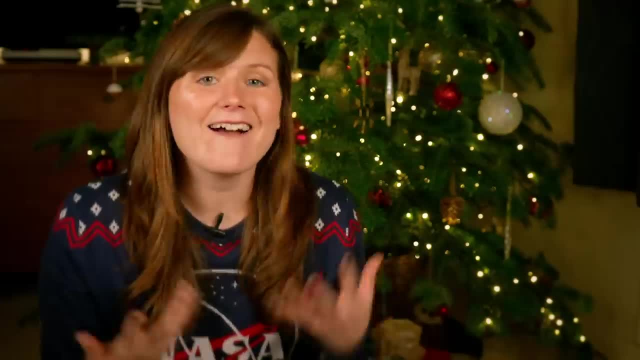 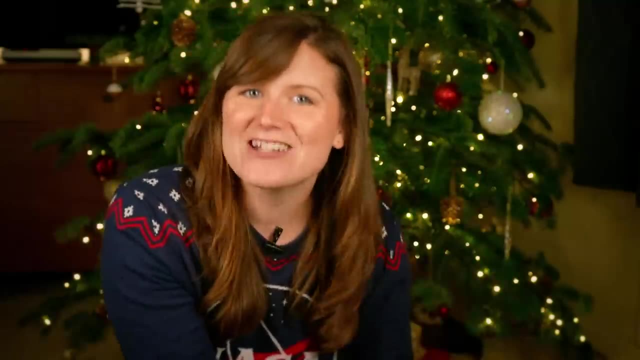 holes in the center that are growing and taking in material, The kinds of things that we know can accelerate these particles up to the huge speeds and therefore the huge energies that we are detecting them with. But there's a lot of these known objects in that big circle region. 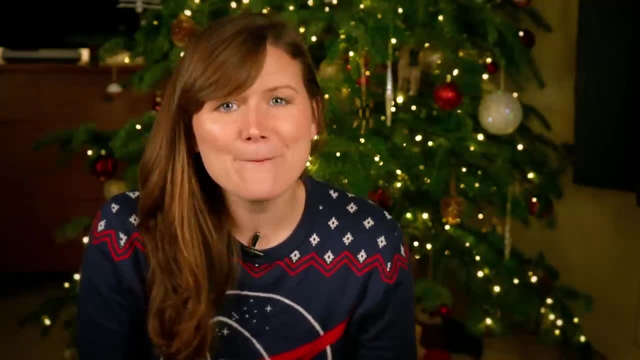 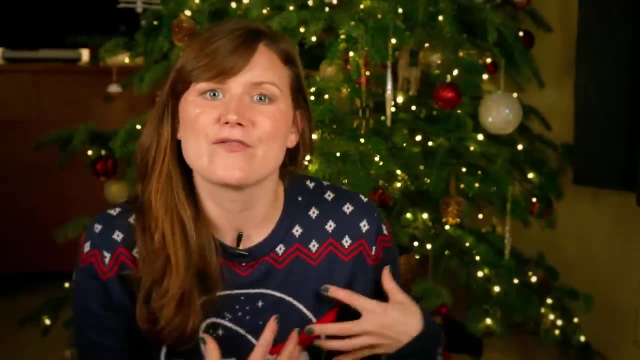 that the event could have come from. Plus, you also have to remember that these cosmic rays are charged particles. So if you're looking at a big circle and you're looking at a big circle of particles, you know if they're a proton or the, you know the nuclei of an atom, then they're. 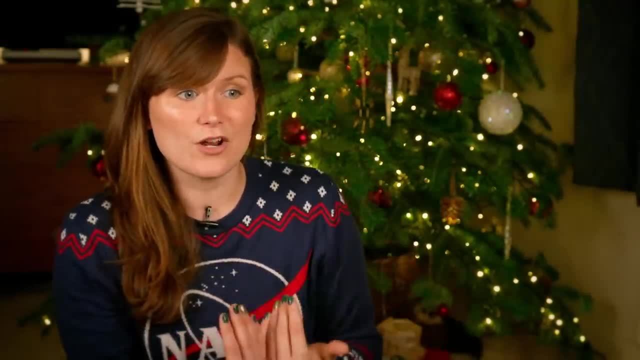 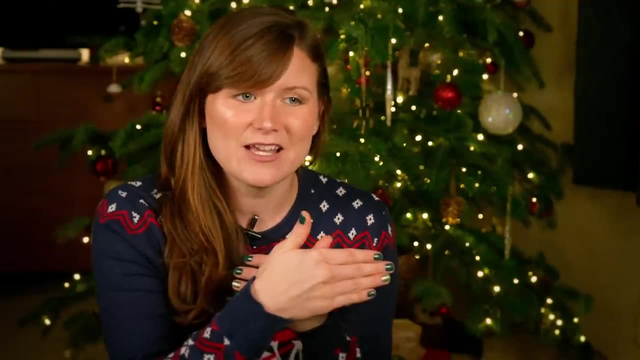 going to be positively charged, which means as they travel towards us here on Earth, they've got to come through our galaxy, the Milky Way, which has a lot of magnetic fields which could deflect them, And then again you think they've come from one direction, but actually they've been. 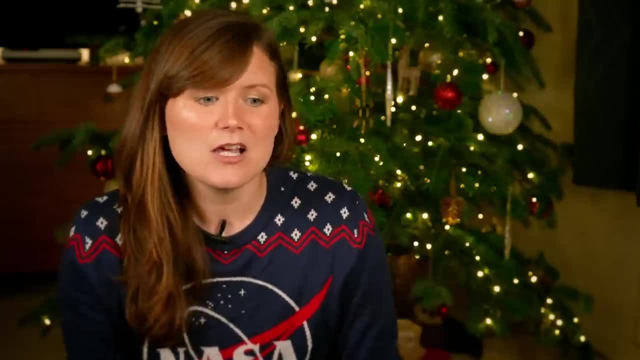 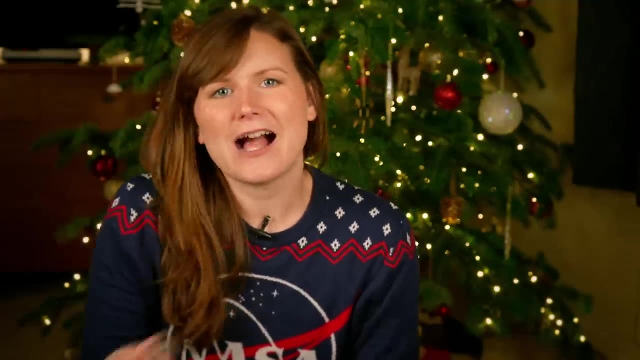 deflected and they've come from over there, which messes up, you know, when you're trying to work out what could be the source of these cosmic rays. Now, depending on how big the nuclei of the atom actually is, you know that sort of the heavier the atom then the more charged your nucleus is going to be So technically, the more it'll be deflected, but then also it'll be heavier, so it'll resist deflection slightly So we can actually model for, if you have a different size, sort of like charged particle, how much is it going to get deflected from these different? 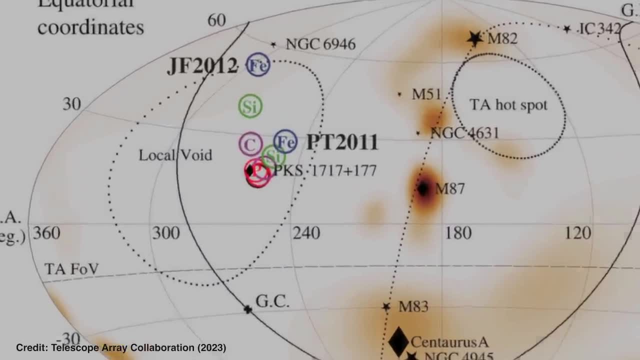 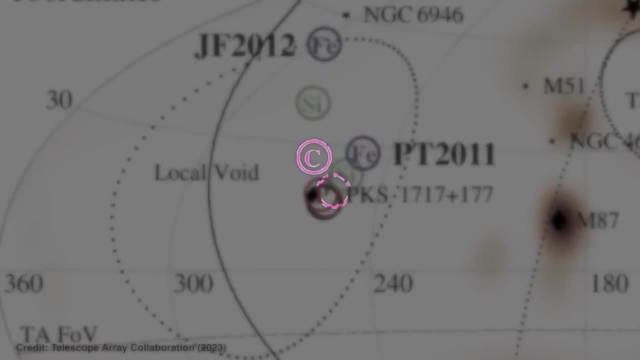 regions. So that's what the collaboration have plotted here. In red is shown where the particle would have come from if it was a single photon. Then in purple is where the particle would have come from if it was a carbon atom nucleus, And then green is. 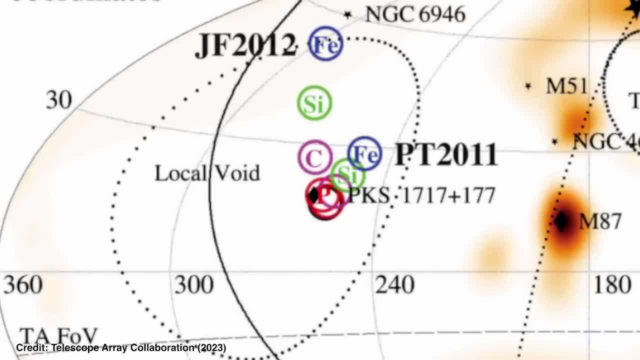 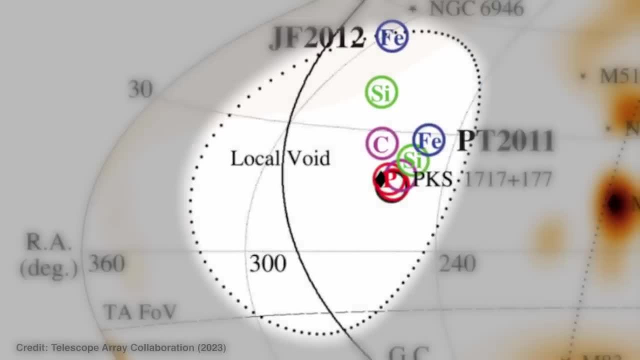 silicon and blue is iron, And so, hopefully, what you can see is that all of these models seem to take the origin of the Amaterasu particle to what's known as the local void, where there's just a dearth of nearby galaxies, just a big chunk of empty space, And while there are background. 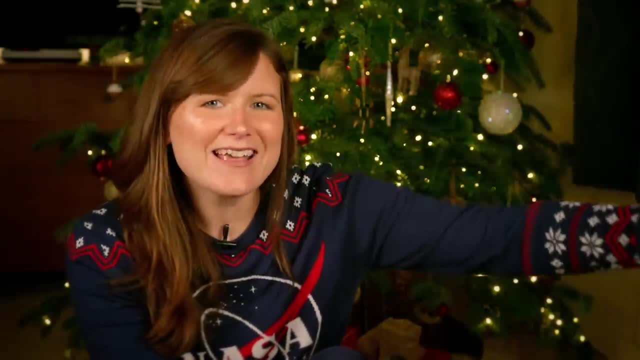 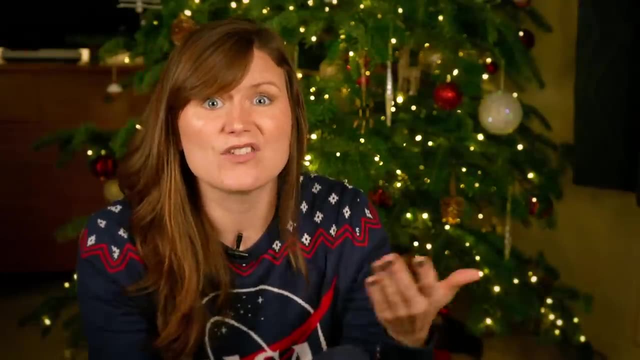 galaxies in that region of sky there are a lot further away. they're thought to be too far away to give you a cosmic ray of the ultra high energies that are in that region of sky That we've observed here, Given the energy of the Amaterasu particle. the collaboration reckon. 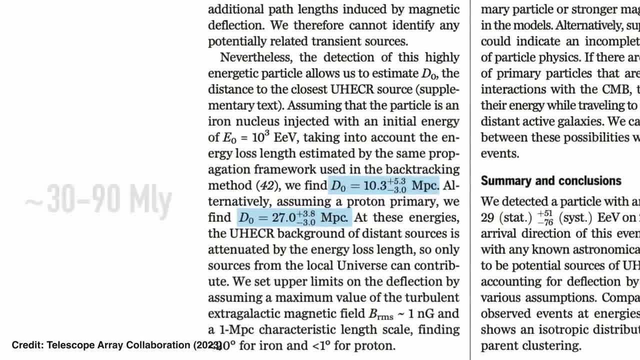 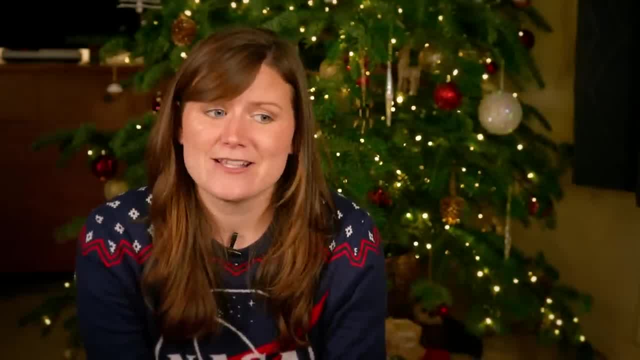 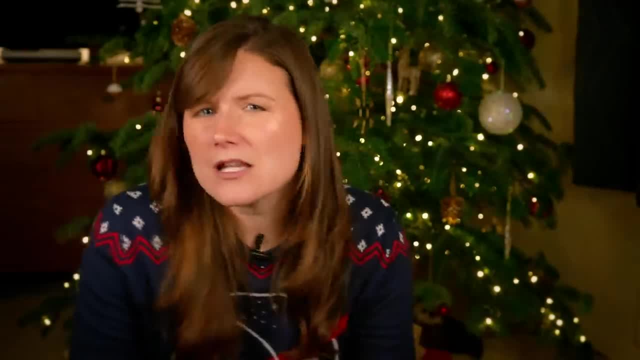 it's somewhere between 10 and 27 megaparsecs away, which is around about 30 to 90 million light years away. So explaining the Amaterasu particle is gonna take some work, because either maybe you know- the Milky Way's magnetic field is stronger than we think, Perhaps there could be. 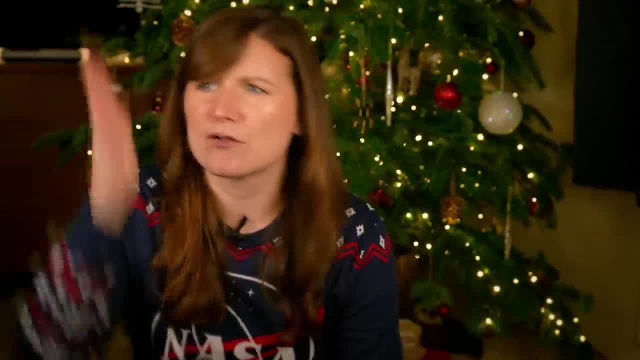 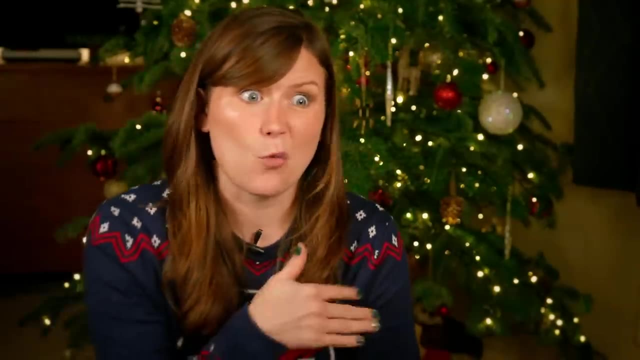 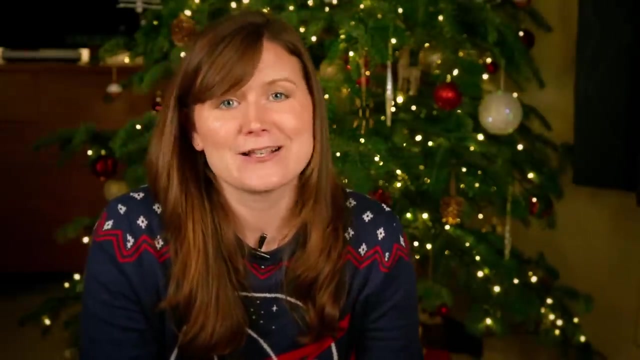 more deflection going on, and therefore it would be coming from a different direction than we've realized. Or there is a source of high energy radiation in the local universe that we're just not aware of at all, Or, as the authors of this paper in the abstract so beautifully put it, we have an 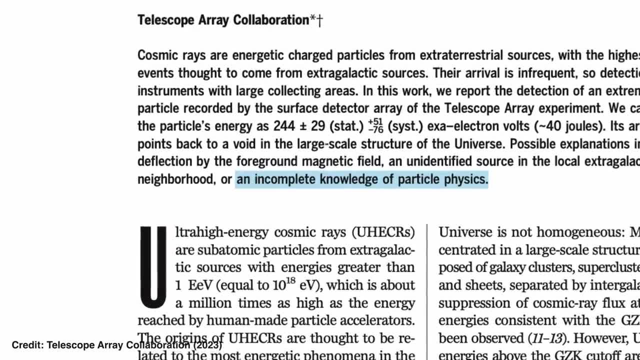 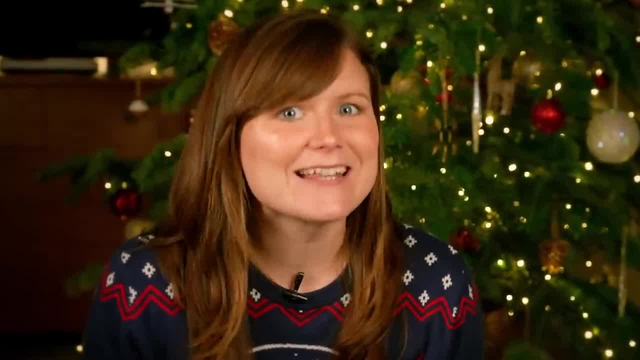 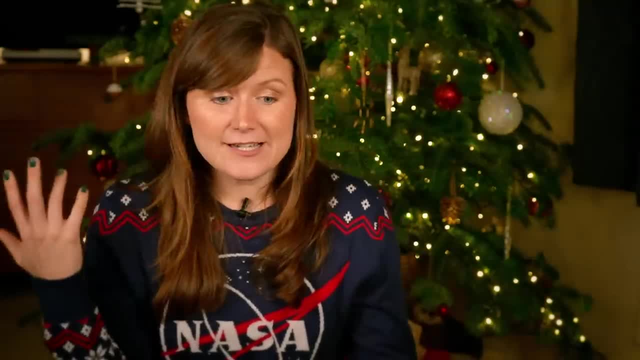 incomplete knowledge of particle physics, So there's clearly something going on here that we don't know about, which I think is a really exciting thought to take us into 2024.. All right, that's it. Thanks for watching. That's it for Night Sky News for this month and for this year as well. Can you believe I've been? 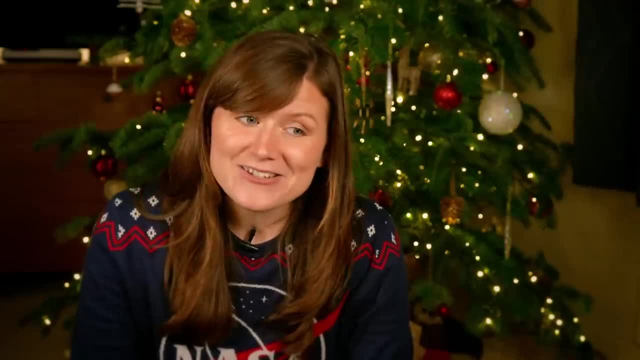 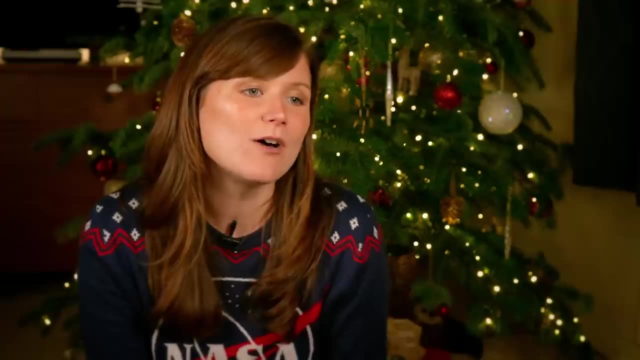 making Night Sky News videos now for five years. So I just wanted to say I am so thankful to all of you who continue to tune into Night Sky News every single month and who share it with friends and with family. I'm so incredibly grateful. Don't worry, Night Sky News is not going anywhere. 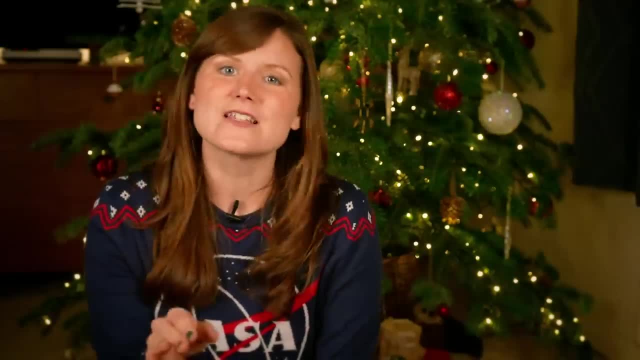 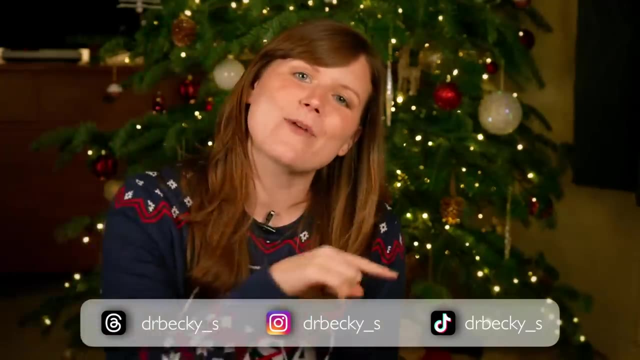 We are continuing into 2024.. So, as usual, if you see any space news stories on your travels around the internet that you want me to cover in a future video, please do so in the comments below, And if you want to see a future Night Sky News video, then send them my way over on social media. 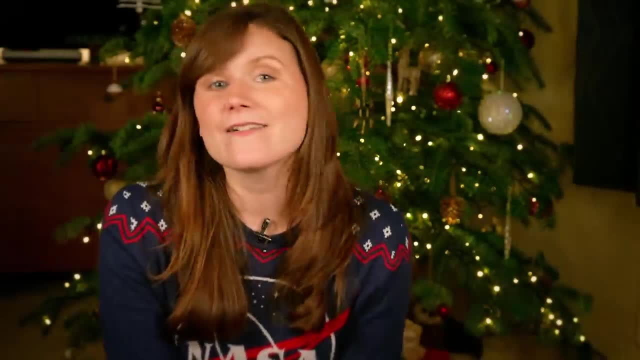 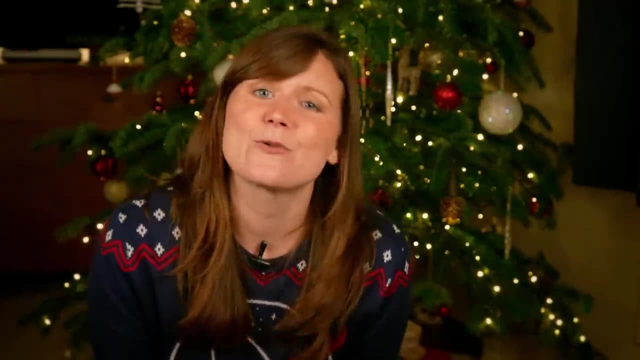 All that's left for me to say is that I hope you all have a very merry Christmas or happy Hanukkah, if you celebrate or if you don't- just a very restful betwixtmas and new year period, But, most importantly, until next time, everybody happy stargazing. 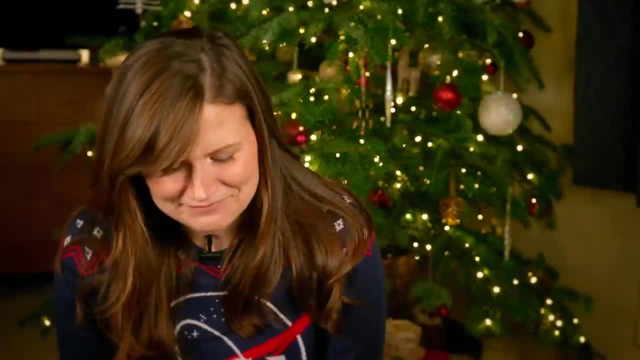 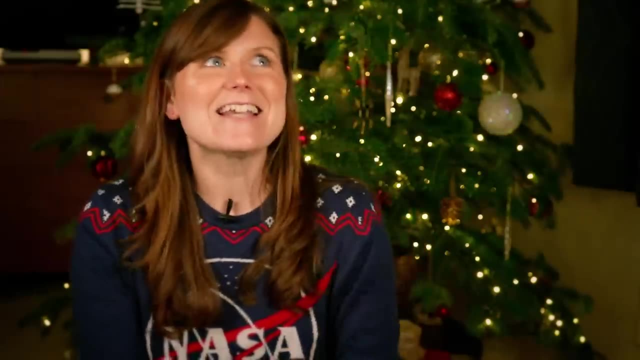 We have officially released, released. We've officially reached. We've not released the solstice. Released the solstice into the world, International space, International space station. I'm gonna get this eventually. Have some juice. Have some juice. that'll make things better.